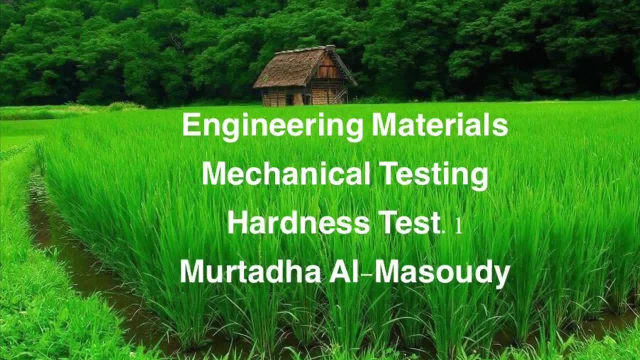 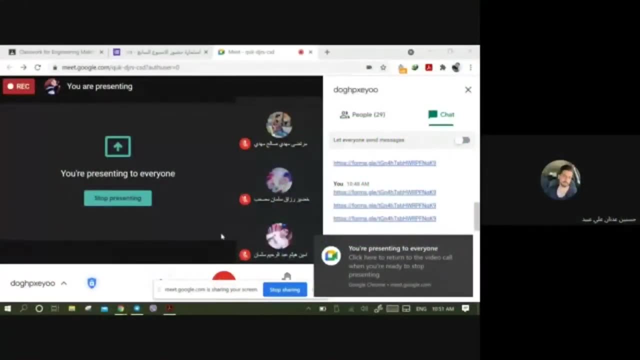 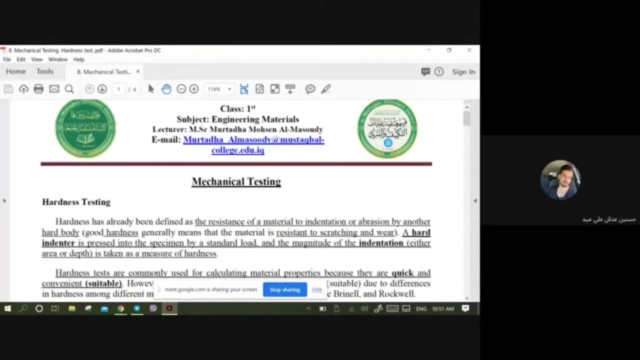 Thank you. This is our lecture, which is today's lecture. It was published yesterday. of course, This is the lecture. The lecture's topic is Mechanical Testing. Mechanical Testing, I mean mechanical testing, Mechanical testing, Of course, the engineering materials that are usually present. 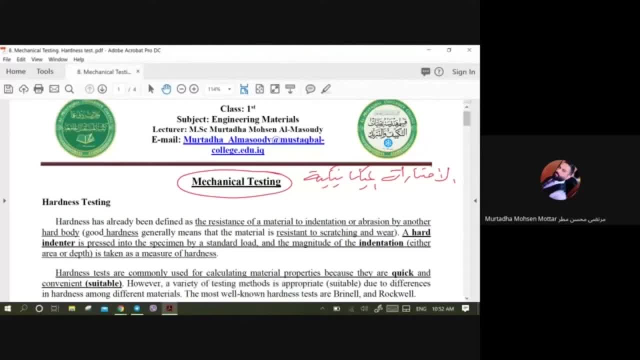 have physical characteristics, mechanical characteristics, chemical characteristics and different characteristics. So I want to know the characteristics of the material, Any characteristics, For example, I want to know the mechanical characteristics. So there are mechanical tests to know the mechanical characteristics of the material. 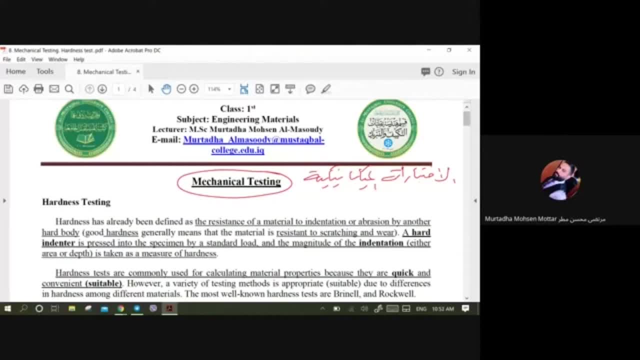 And I want to know the physical characteristics Also. there are physical tests to know the physical characteristics of the material as well as the mechanical characteristics. Here in the engineering materials, as engineering materials, I will focus on the mechanical tests. I have a set of tests, not one test. 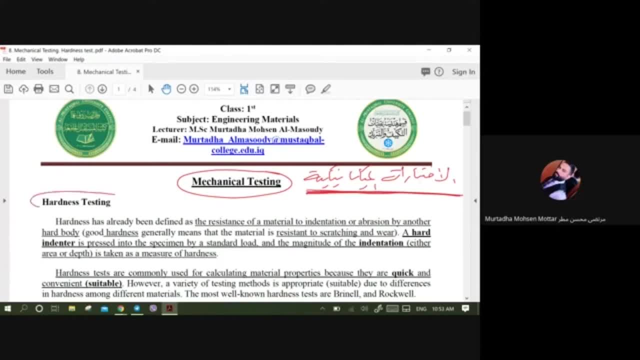 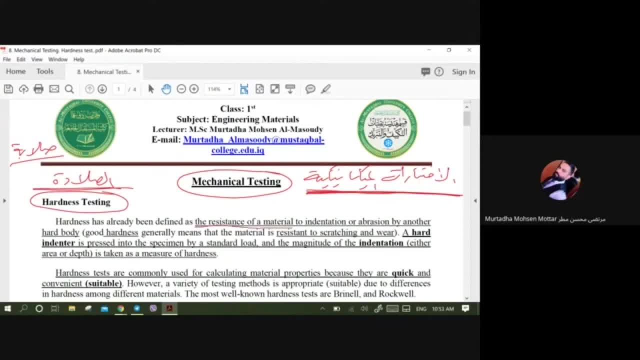 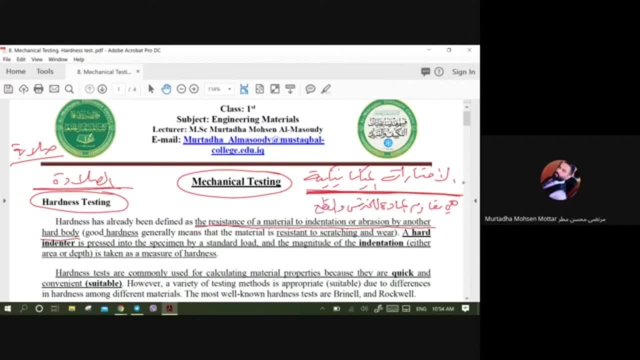 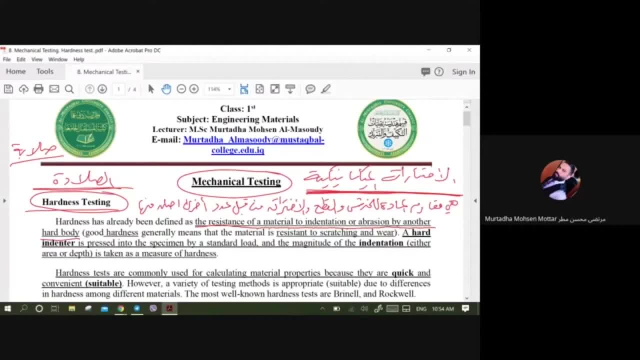 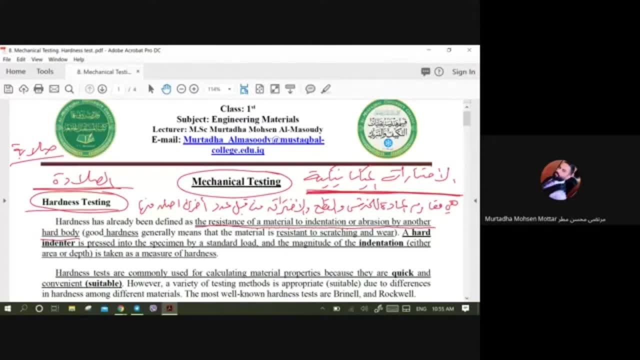 Iron. because? why? Because his prayer is higher. Therefore, as a definition, the resistance of the substance to cutting, breaking and breaking by another number is stronger than it. So if you see the word good hardness, which means a good prayer, it means the resistance of the substance to cutting and breaking and the resistance of the substance to cutting and breaking, which means trouble, 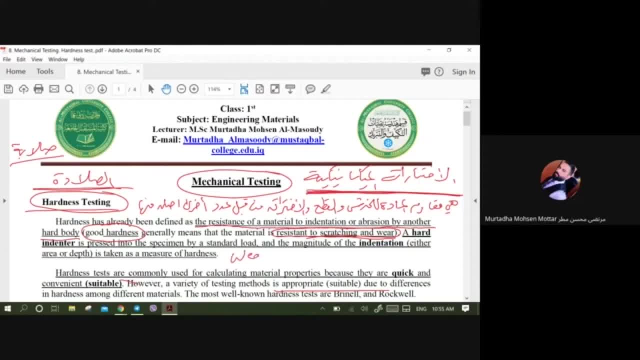 In order to know what the word break means. what is trouble? Trouble is, when I say a substance that breaks, that is, a substance that removes a piece from it. What does this mean? If something happens to you physically? or both of them move one relative to the other, or both of them move one relative to the other, or both of them are equal. 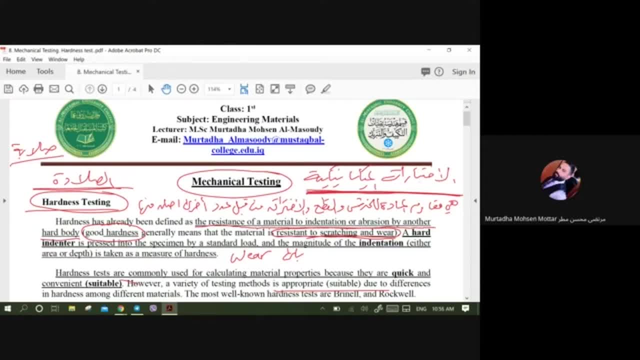 then it is possible that a piece of one of these two substances that is less solid will be removed. Why? If you see a disc brake rotor, which I call the discs of the car, you see them. of course, we saw them. 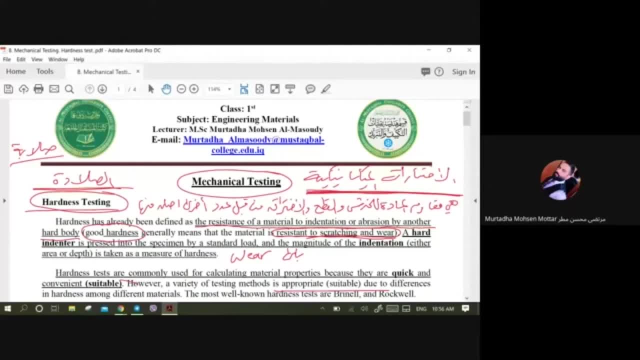 After a while You can see. what they do is that either they are replaced or that a piece of them is used to break the structure of the saw, Why A piece of one movement is removed from the other due to the destruction of the latter. so it is called a disc. 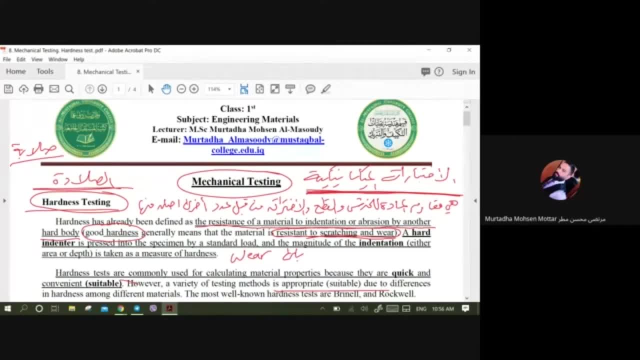 In order to avoid forgetting what a disc means. this instrument is called a disc, So here in prayer, I have two terms that I need to know. These are the two terms which I have to learn. The first is the term of a person who is a member of the group. 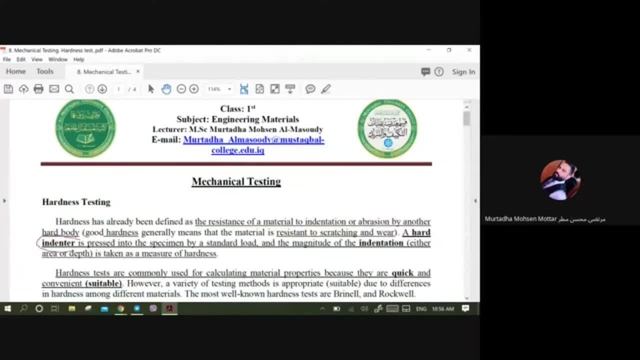 I have two terms that I need to know. The first term is IDENTER and the second term is IDENTATION. In this test, these two terms are very important. This year I focused on them and brought them to the test and told them to come out with important things. 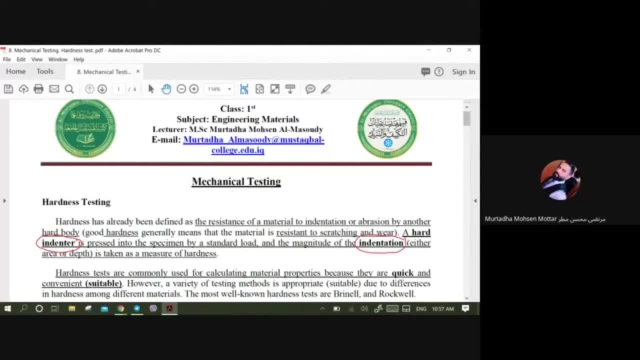 I brought them to the test and they didn't answer. I brought them to the test and they didn't answer. More than 80% of them didn't answer except for a small number. Now I want to tell you that you have to focus on the important things. 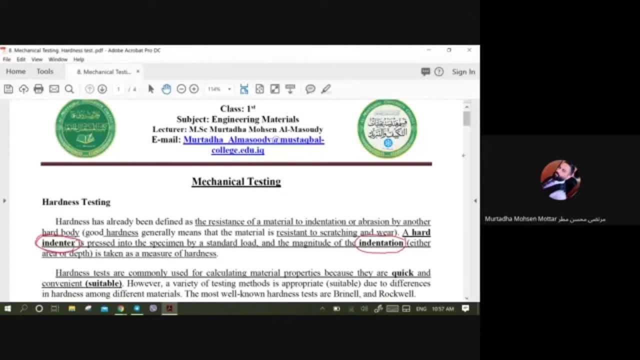 I want to tell you the difference between IDENTER and IDENTATION. Of course, this N does not mean indenture, but IDENTER and IDENTATION. IDENTER, as a definition, is the number of numbers used to measure the strength of a person. The number of numbers used to measure the strength of a person. 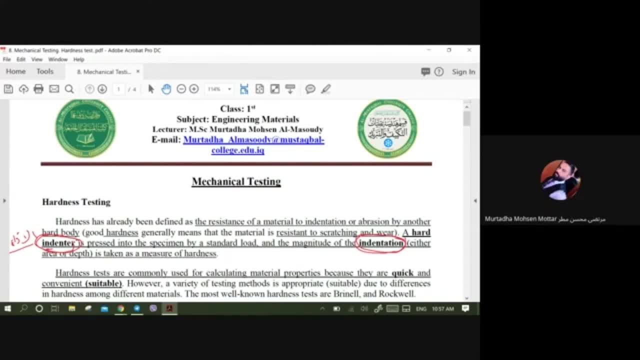 I call it IDENTER. If you ask me what is IDENTER? IDENTER is the number of numbers used to measure the strength of a person. IDENTATION is the effect that the tool leaves on the eye. IDENTATION is the effect that the tool leaves on the eye. 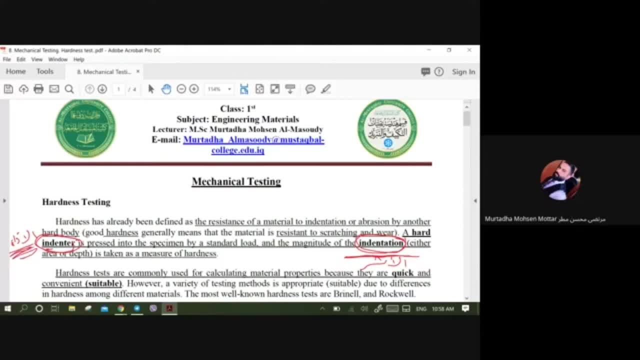 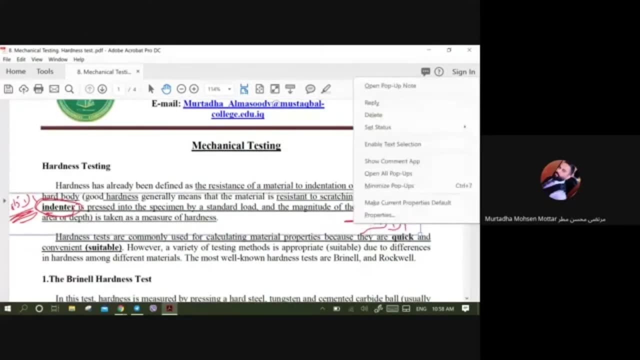 So now you have IDENTER and IDENTATION. You have to differentiate between them. These are very important things. Now, this test, which is the prayer test. It has two important features. First, it is quick. This test is quick. Second, it is suitable. This is the second point. 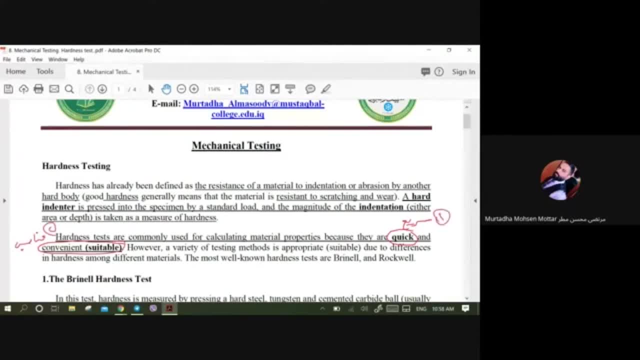 The first point is quick And the second point is suitable. This test means that I can run and get results in seconds. I can get results in seconds. I can get results in seconds While there are other tests that take hours or days to get results, While there are other tests that take hours or days to get results in seconds. 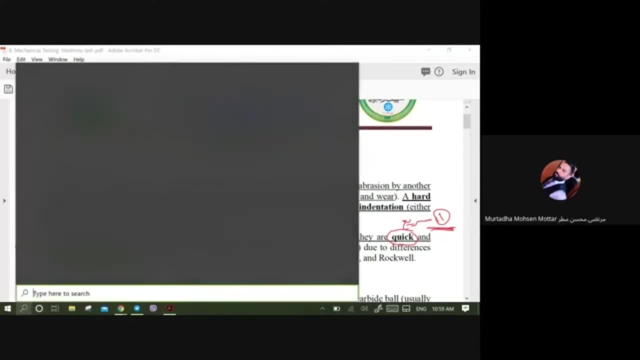 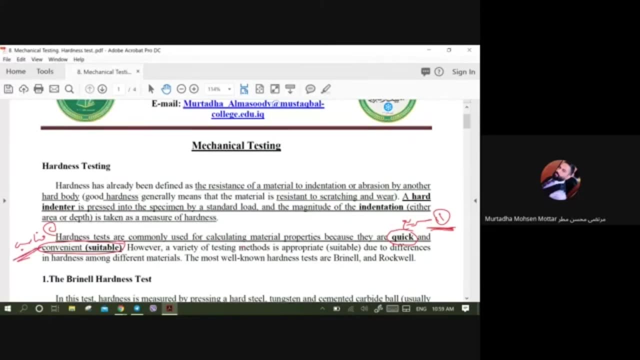 So this test is quick. Second, it is convenient. I say convenient. Why is it suitable? Because I can know the mechanical characteristics of the material through this test. Because I can know the mechanical characteristics of the material through this test. Because I can know the mechanical characteristics of the material through this test. 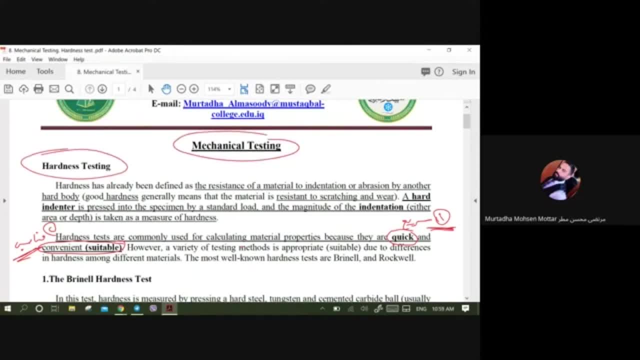 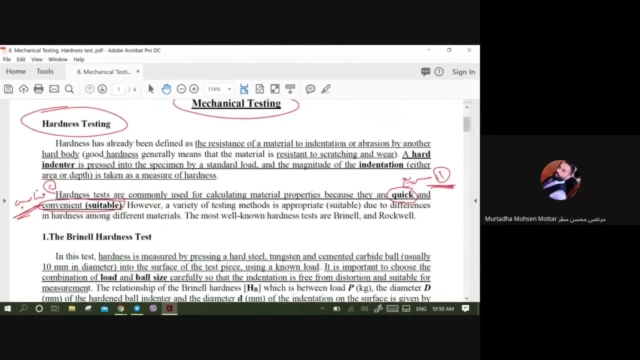 Of course, there are ways to test the prayer, Not one way. I have a set of ways, I have five ways. I will take only three ways And today I will take only the first way. Today, I will take only the first way. But why is it different? 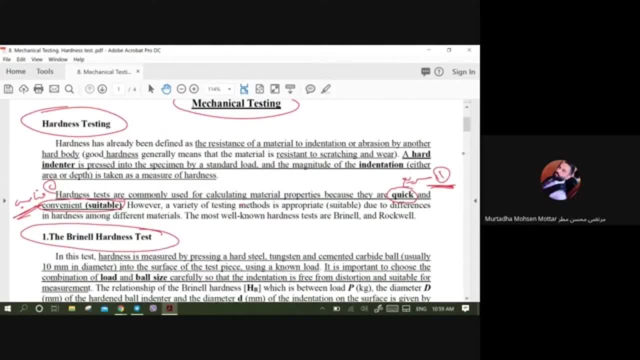 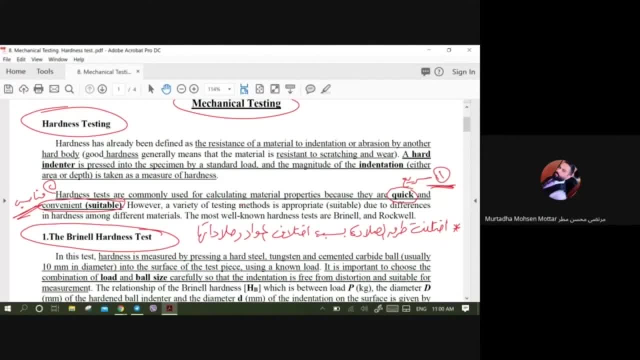 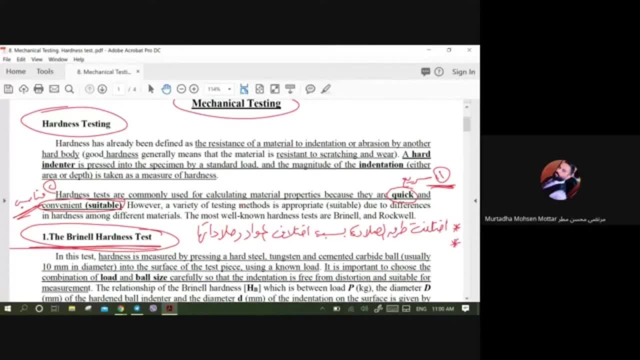 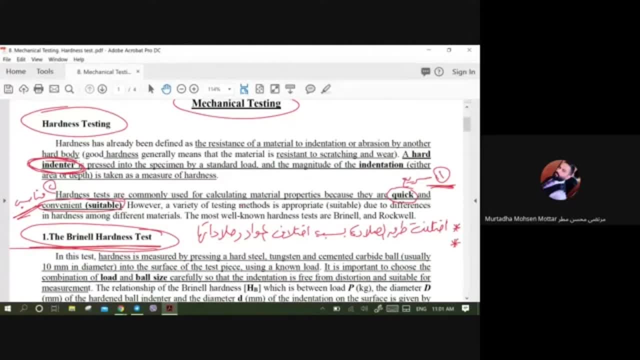 And the second type, as you can see, is the definition of solidity, the resistance of the material to wear and tear and the penetration by another number of them. Now, here we have a difference between identity and indentation, these two: Identity is the tool used to measure the solidity of the material and indentation is the effect of the tool on the eye. 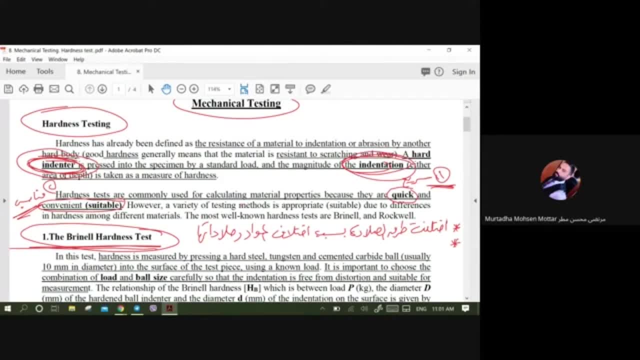 Here we have this test, the test of solidity. as we said, a quick and suitable test, the most important of the two, And you have different types of solidity due to the difference in the material and solidity. What is the difference between one method and the other? What is the main difference? 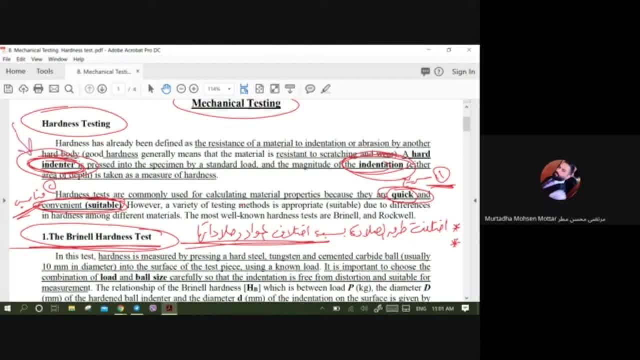 The main difference is this: indentation, which is the tool or the tool used to measure the solidity of the material. Identity is the tool or the tool used to measure the solidity of the material. Identity is the tool or the tool used to measure the solidity of the material. 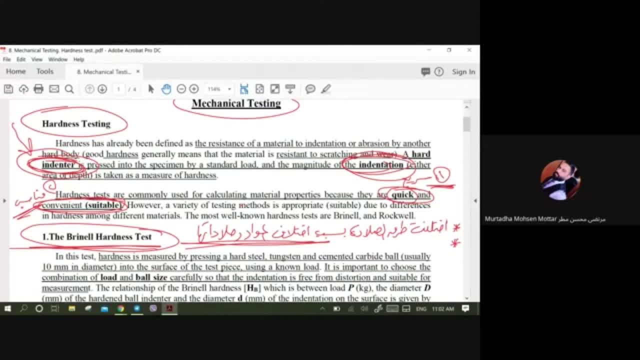 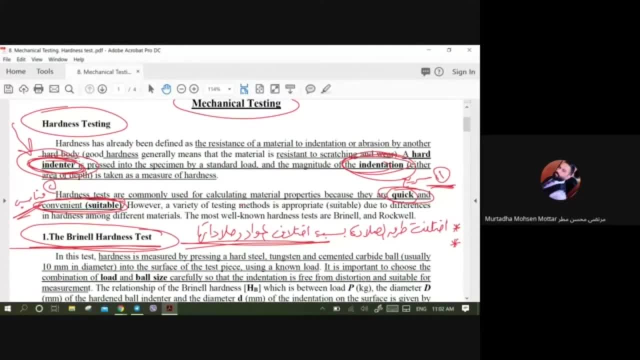 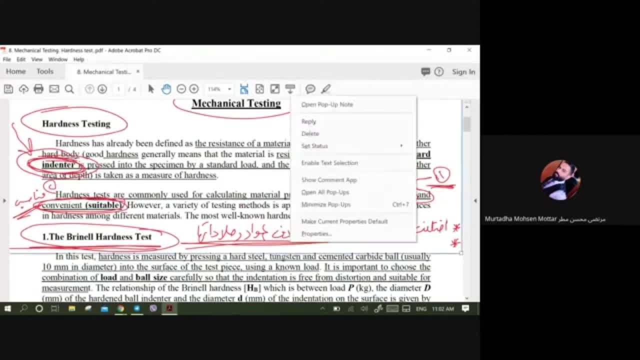 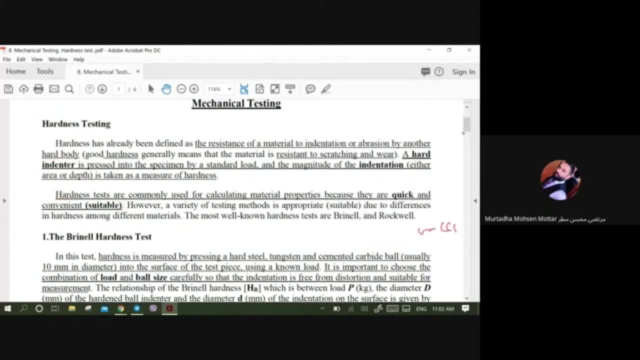 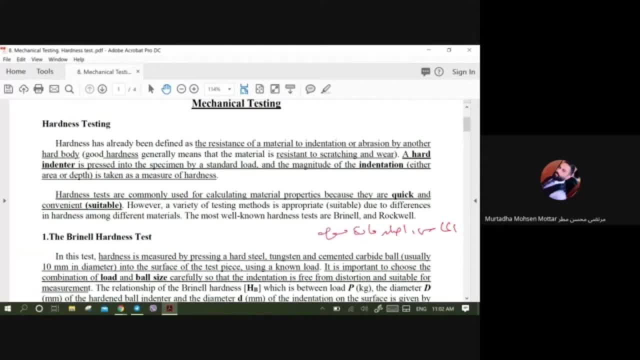 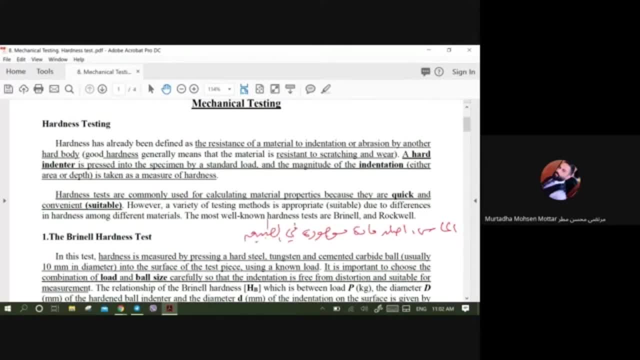 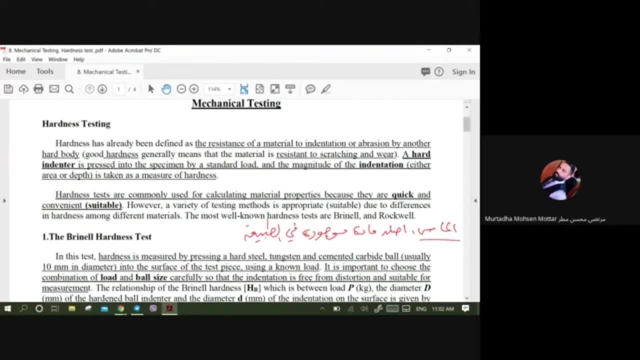 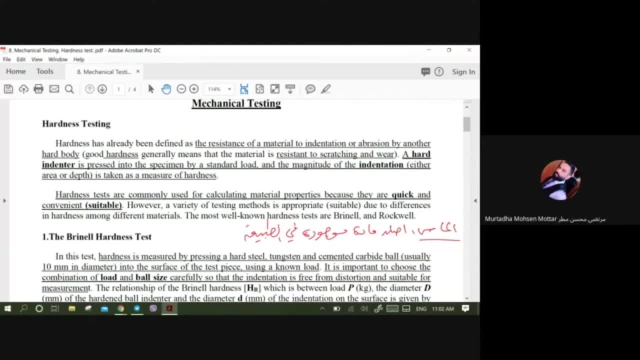 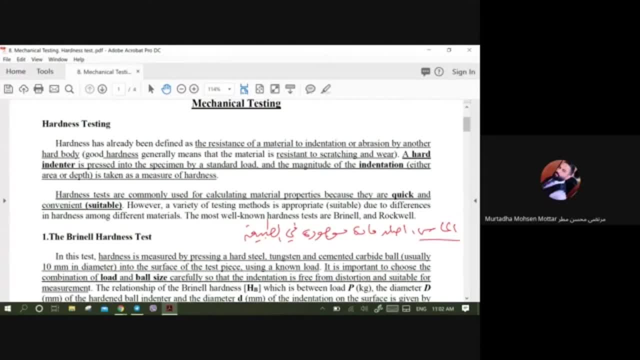 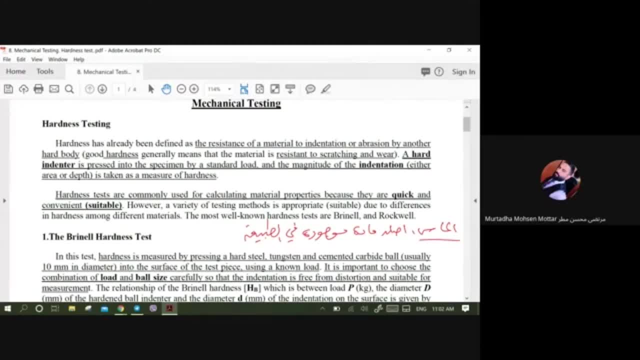 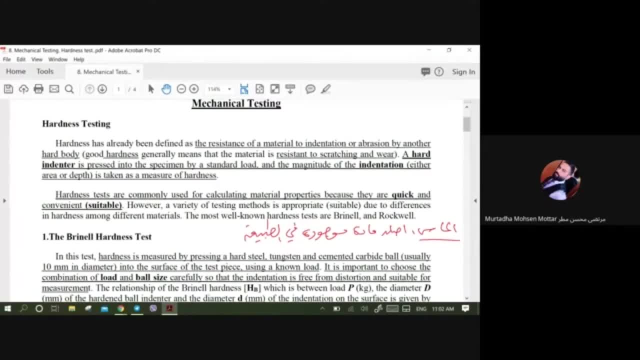 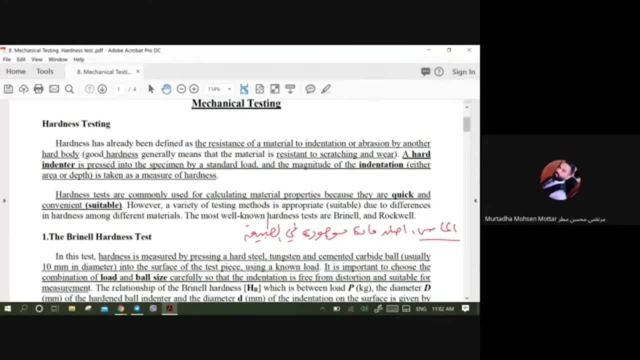 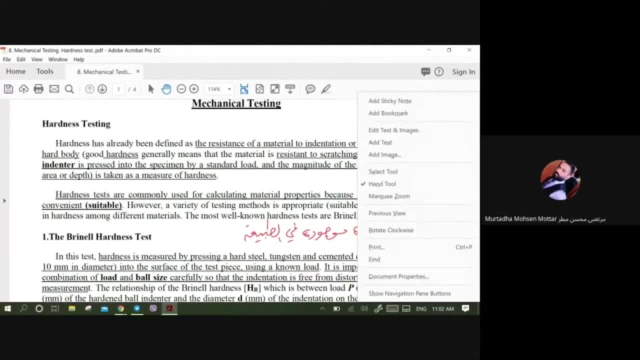 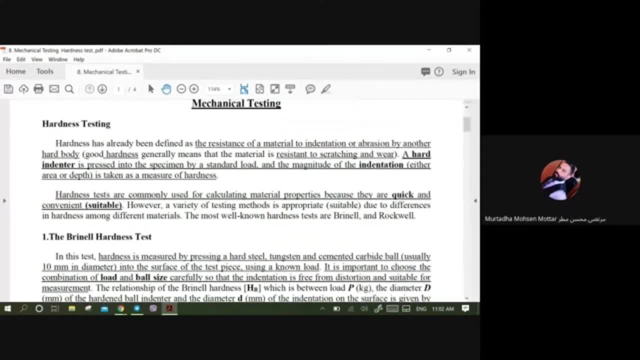 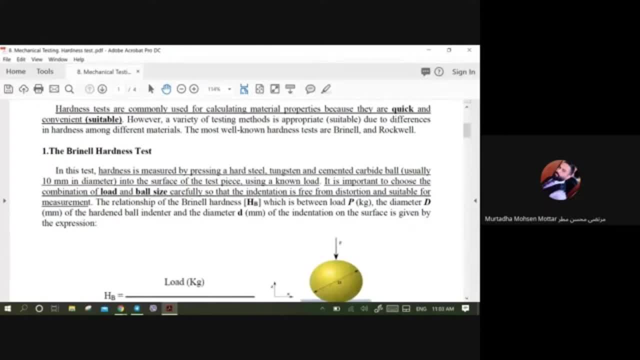 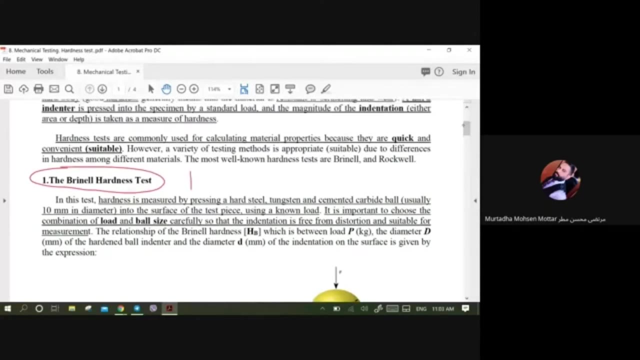 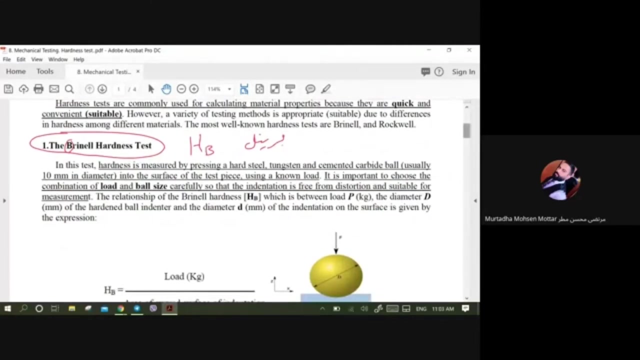 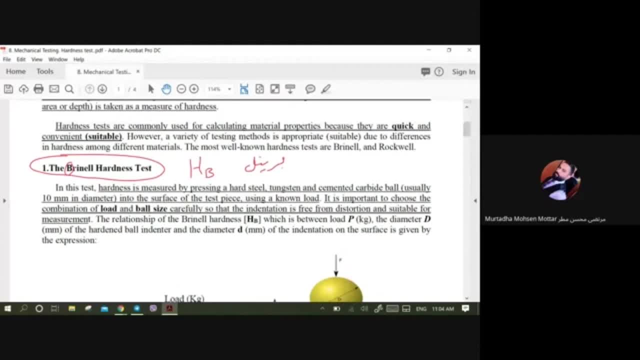 In this type of test, the tool used is either hard steel ball made of steel, or tungsten or cemented carbide. Of course, steel is tungsten, tungsten is tungsten. cemented carbide is carbide cementite. 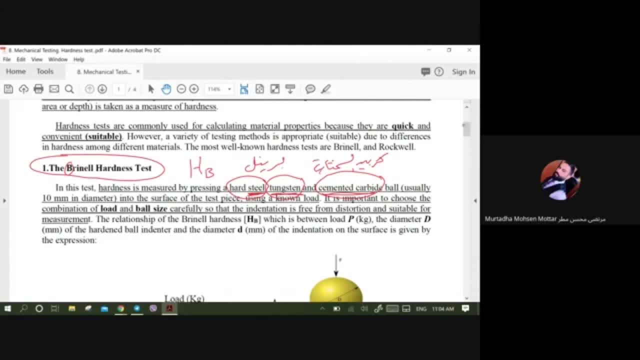 Carbide, Carbide cementite, which is the symbol of Fe3C. this is the symbol of it. this is a very high-strength material, so in this type of test you use a ball made of steel or tungsten or cementite carbide. 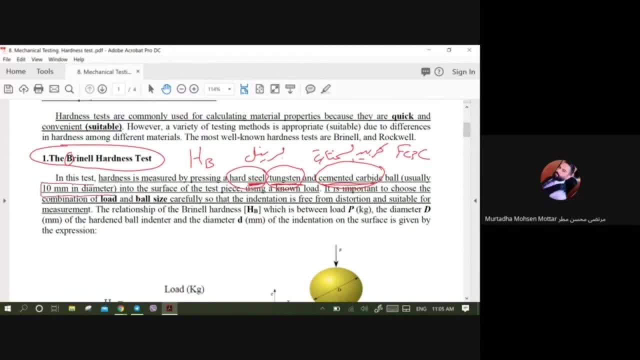 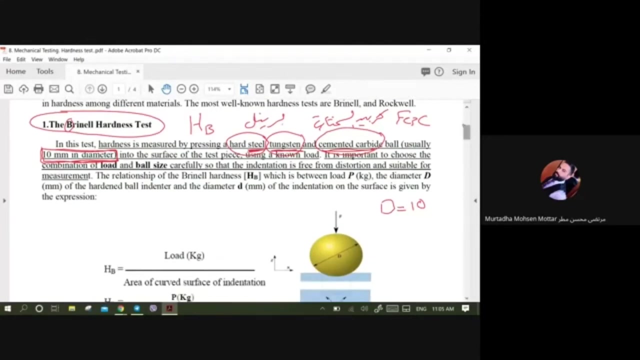 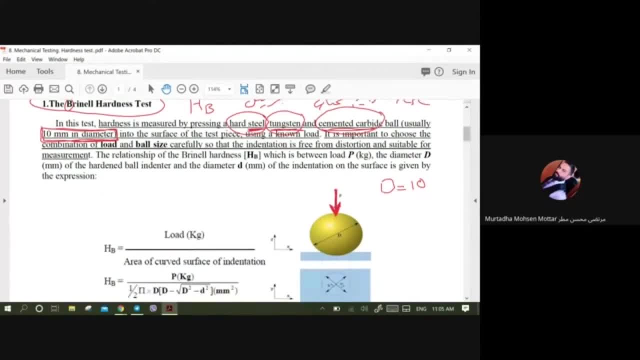 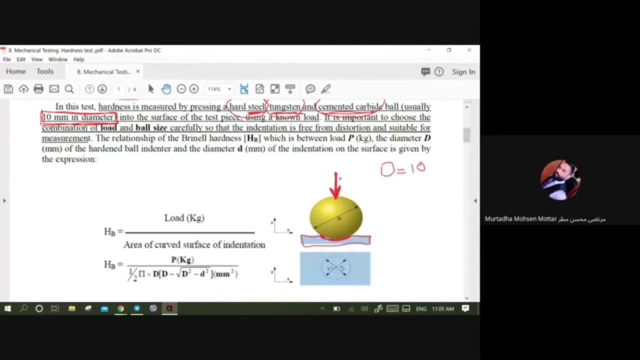 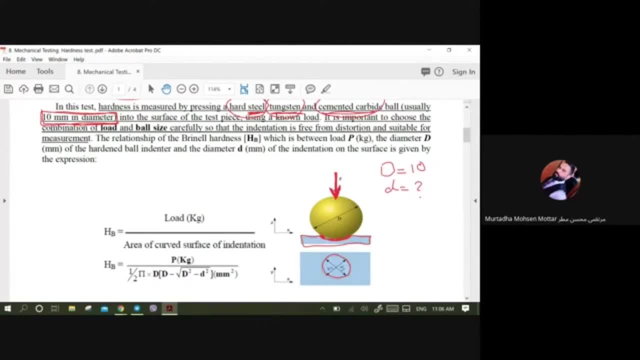 For the effect there is a specific line. D is the capital and the ball line is 10. If you don't give it a value, you assume it's 10, and if you give it a value, you use that value And D is the effect line. when I press the ball with a certain load, it will leave an effect. 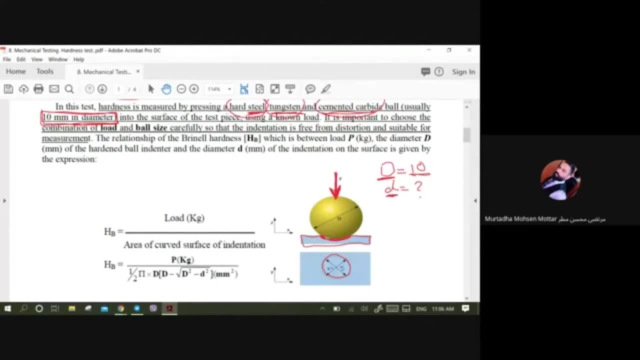 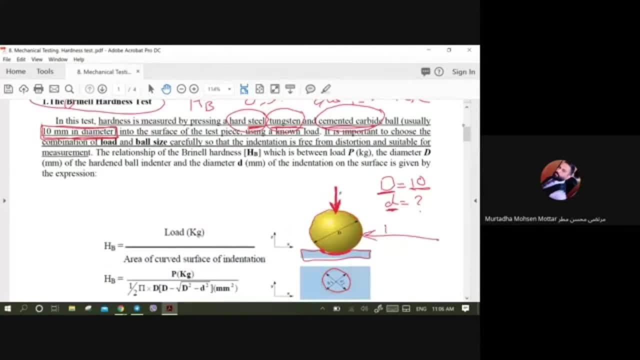 This is the effect line. D is the effect line. I don't have a ball here. I have a tool here and I call this tool the IDENTER. I told you a while ago that the tools used to measure the value of the material are different. 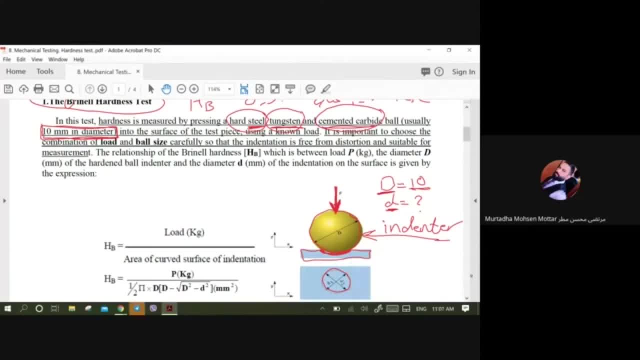 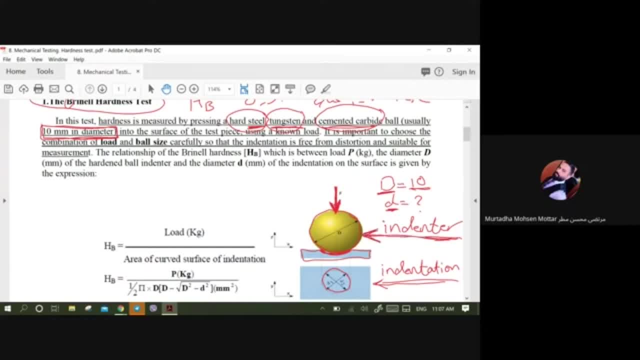 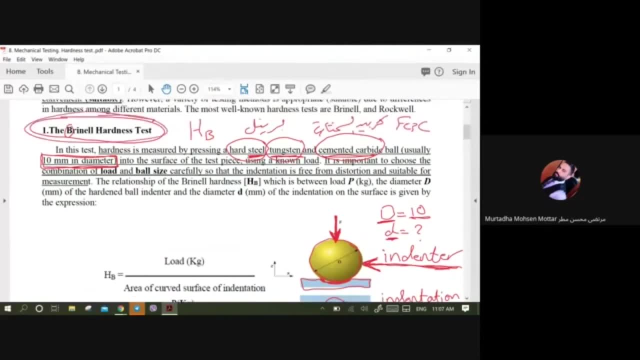 IDENTAR is the tool used to measure the value of the material, And the tool here is a ball. but you have to pay attention: This is the first type, which is BRINAL. When we go to the second type, it doesn't use a ball, it uses other tools. 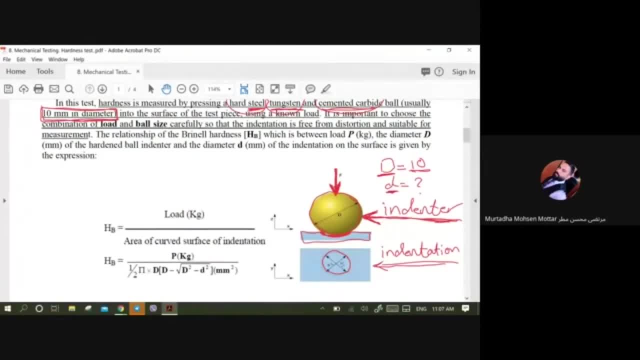 That's why I didn't say the ball used to measure the value of the material. No, I said the tools. regardless of the type of the tool, It can be a ball of a certain type. second type is a BRINAL. Third type is a BRINAL. 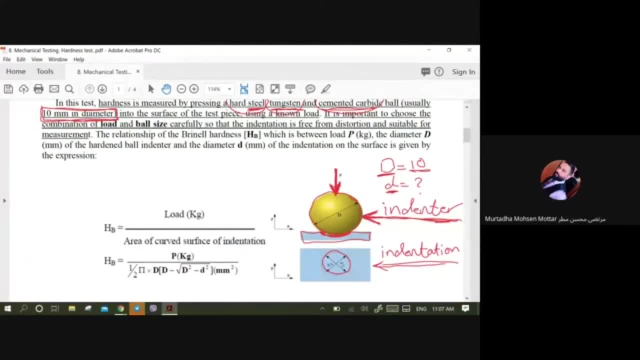 Therefore this is different. so I said IDENTER. The tool is not defined. the tool is used to measure the value of the material. IDENTATION is the effect that the tool leaves on the sample. Also, I didn't say that the ball leaves on the sample. 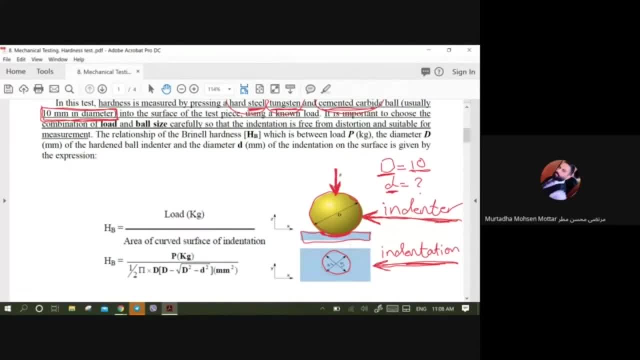 No, I said the effect that the tool leaves on the sample, Because this tool can be a ball, it can be a BRINAL or it can be a BRINAL. Therefore, here we said, the tool leaves an effect. After that, when I put this ball, when I put it on the metal, 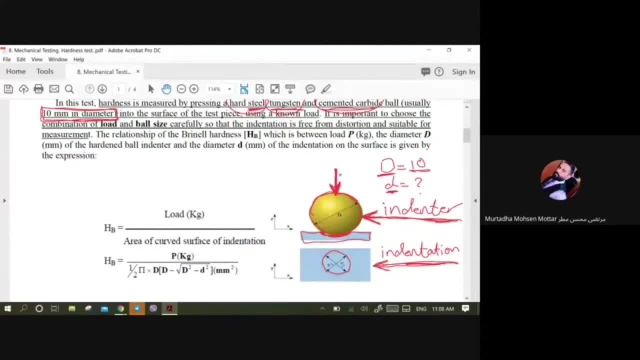 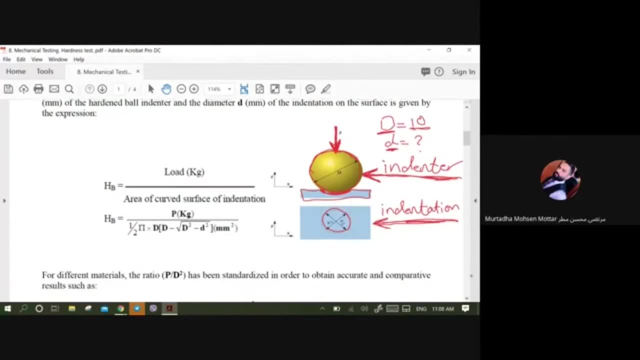 And I put it on a certain weight. it will leave an effect After that. how do I calculate the value of the solid? How do I calculate the value of the solid of this material By this law? This law is the solidity of the BRINAL. 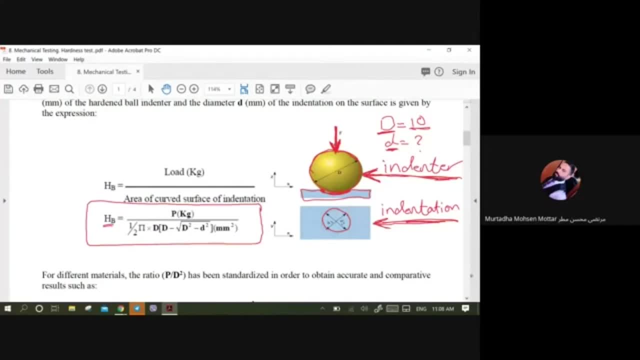 H is hardness and B is BRINAL. What does it equal? P means the load. See in kilograms The force or the load that I use. The weight that I use Here is the load On this half. here you have half And this pi, the constant ratio of pi. 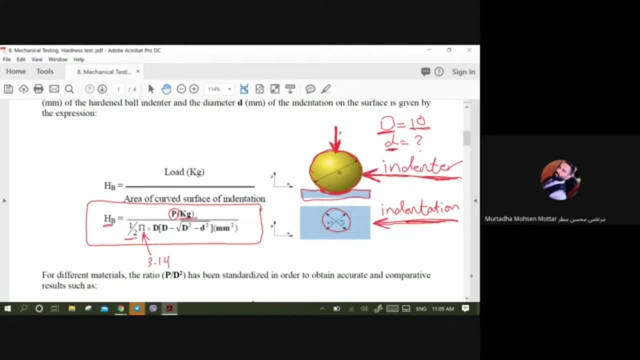 Which is 3.14. Here is the D capital. I open a curve D capital, minus D capital, plus minus d small Plus d under the bridge. So this D capital is the ball's radius. I told you the ball's radius. It can be 10 if you don't measure it. 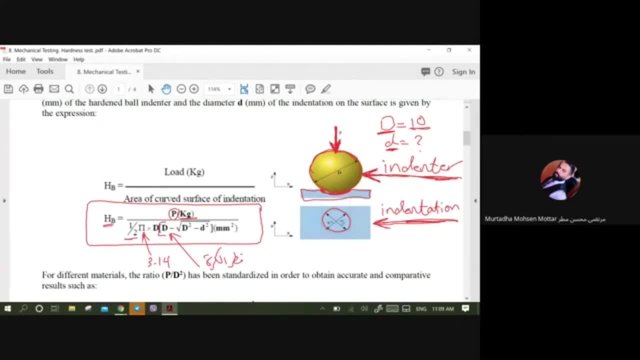 And if you measure it, you use the value that you measure it. This d small is the ball's radius. What is the momentum of the ball? The momentum of the ball, That is the ball's Beck'sgression, The work of tutaj. So what about this one? 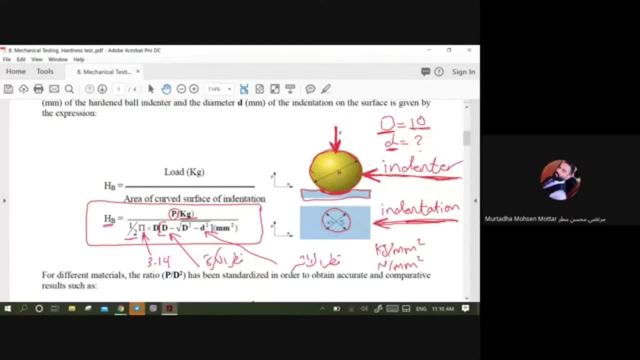 The work of tori. What is the work d הפ? What is the work of Tη Ε중? What is the work of 3.14 Infrastructure? Here the weight will be the units of kilograms per meter per square millimeter. 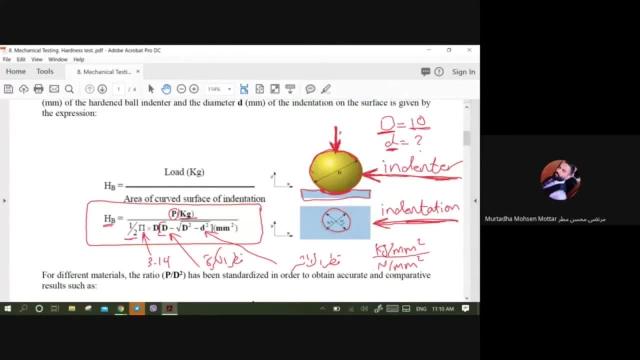 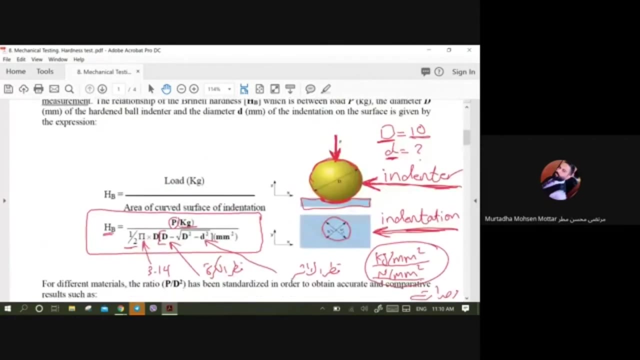 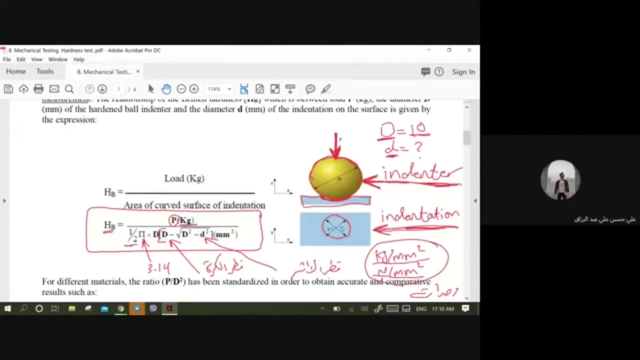 But if we take the units of power per newton, then it will be newton per square millimeter as units. The result we get must be written in its unit by this law. Now here there is a student's question About the law and the laws of the law and the law of the law. 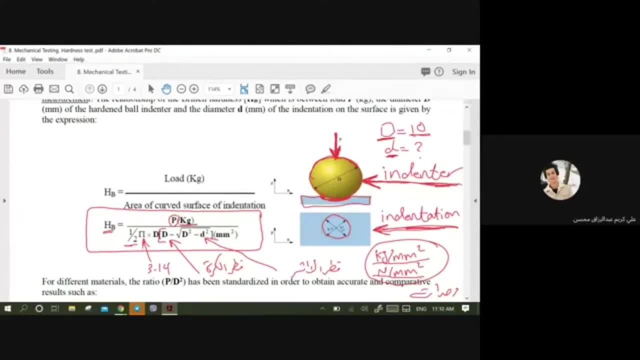 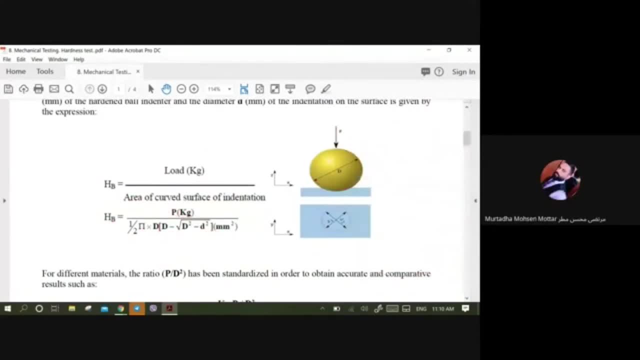 If I have a question, What is the law? The law, The law. I'll go back to it. The law, this is the law of the law. I want you to have the HB, the Brinell's law. I give you the value of P, I give you the value of D capital and I give you the value of D small. 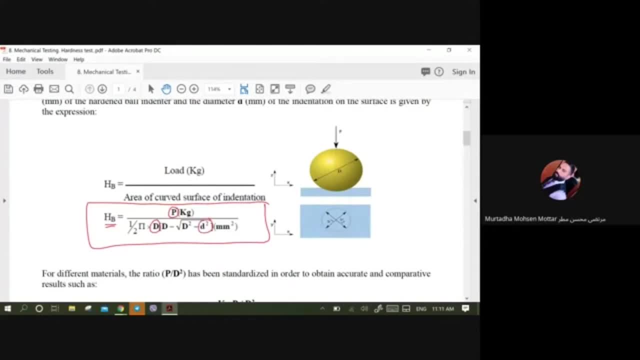 So, as soon as you come to the table And you get the result, as you know, here is the P, the units of kilograms- the position you have is half. you get half the Pi, the constant ratio. who knows the constant ratio, which is 3.14, D- this is the line of the ball. this is the line of the ball. D, capital and D, this small, is the line of the effect. 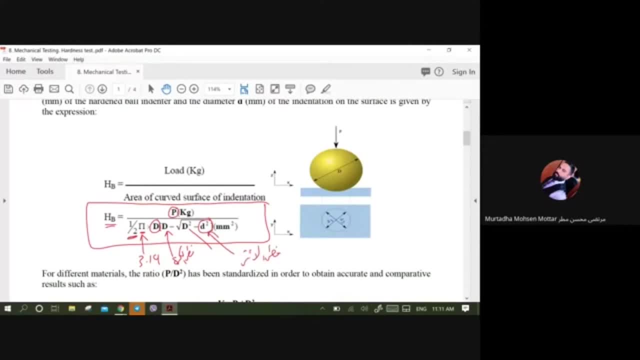 And then I give you here, of course, I give you here with the question, so you just get the result. And then I give you here, of course, I give you here with the question, so you just get the result, And you write the units of kilograms on the square millimeter, or Newton on the square millimeter, depending on the value of the force. 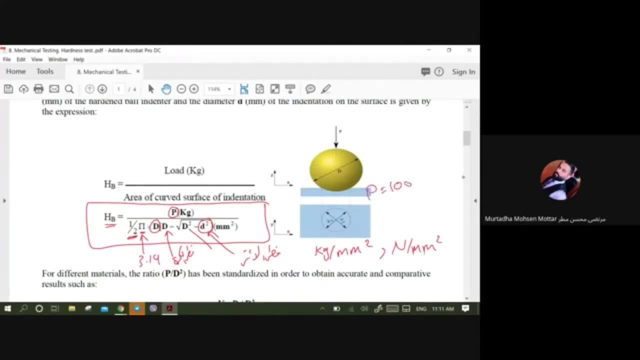 The force, for example. I give you the P, for example, 100 Newton, so the units must be like this: And if I give you the P in units of, for example, 10 kilograms, then the units will be in kilograms units, like this: 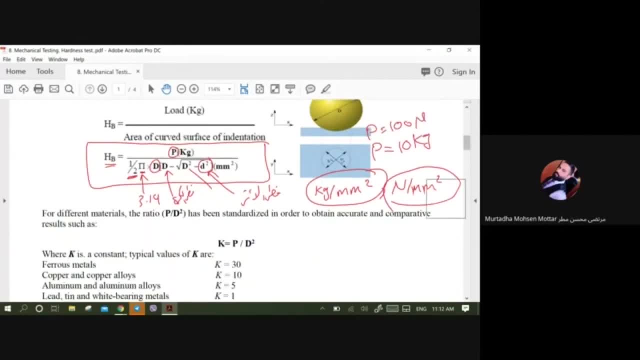 So this is the law. Now, Sometimes something is equal. we are not given D. look, as you can see here in the drawing. look, the effect is proportional to D1, and it is proportional to D2,, as you can see here. 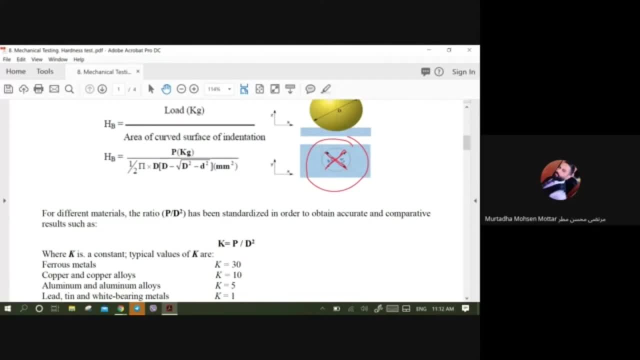 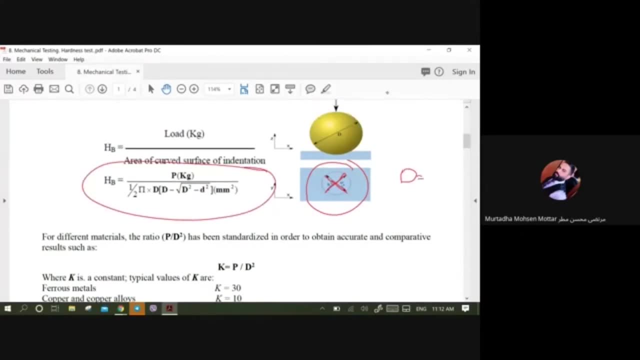 So when you are given D1 and D2, I mean you are given. you see, you are given D. you are supposed to see this law. to solve it, you must have the value of D 10, and the value of D small, let's assume 3.. 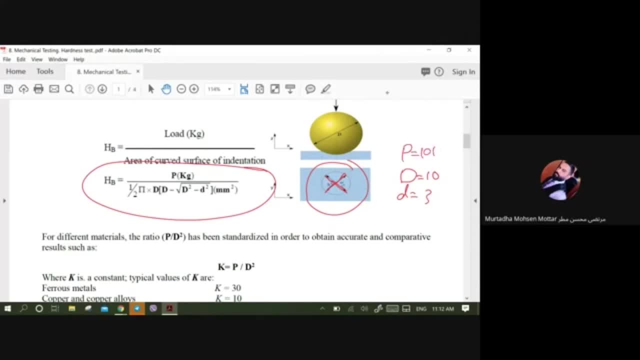 And also I give you the P, for example 10.. So this is the matter. Kilograms, So these three are the p value and the D capital and D this is to compensate them here with the law and to take the value of HP. 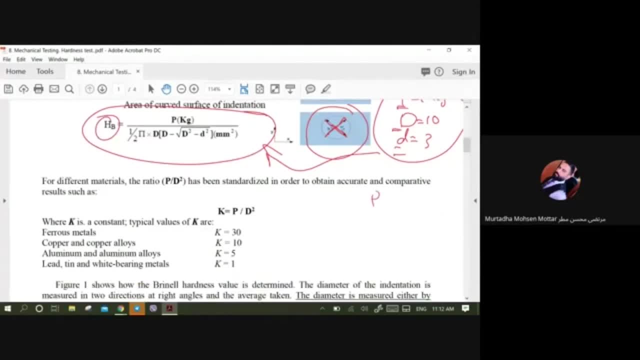 But sometimes, for example, d, gives you the P, for example 10 kilograms, And gives you the D capital. gives it to you, for example, 10 millimeters, And gives you, for example, D1, 4.. 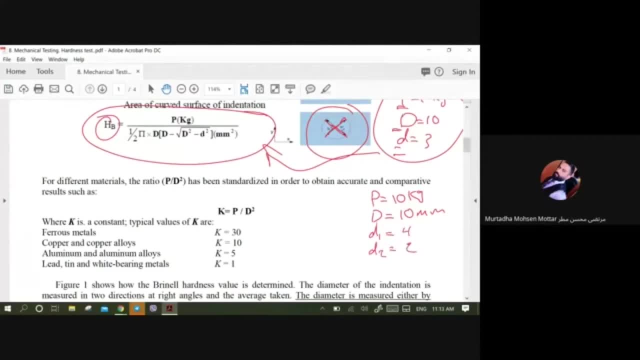 And D2,, for example, 2.. So in this case, what do we do? D1 and D2, you have to take their averages and subtract D. What does D say? D1 plus D2 divided by 2.. 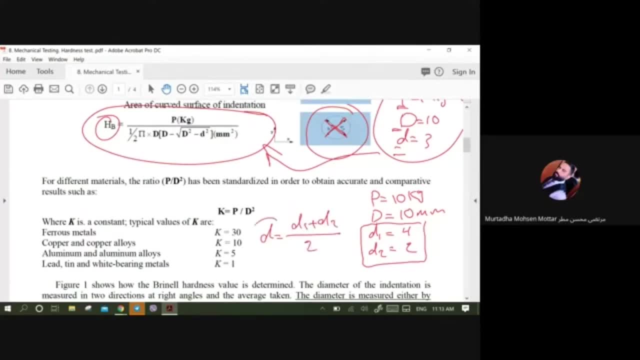 So you put them together and divide them by their number, so you can subtract D. It doesn't replace 4 and 2, no, Here you have to put them together and divide them by 2, so you can subtract their averages. 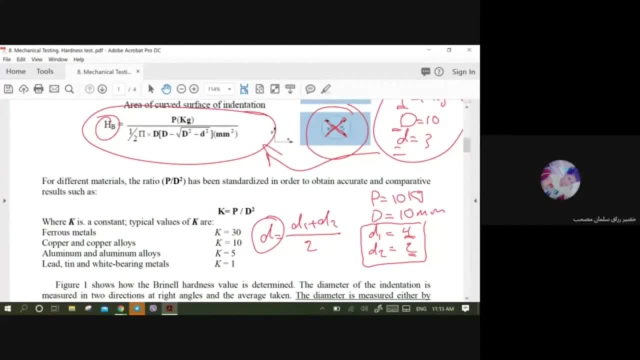 10 plus 10? What is 10 plus 10? D1 plus 10 and D2 plus 10.. Are we going to divide them by 2? Yes, but here I'm going to give you 4 plus 2.. 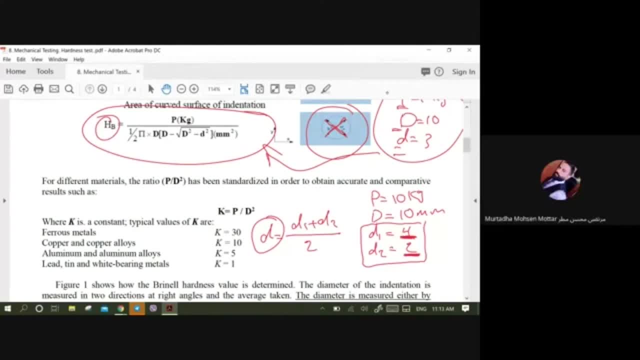 D1 is small. D is small, not D capital. D capital is the size of a ball. As for 10, you have to subtract it. D is small, which is the size of an arrow. If you subtract D1 and D2, you have to put them together and divide them by 2.. 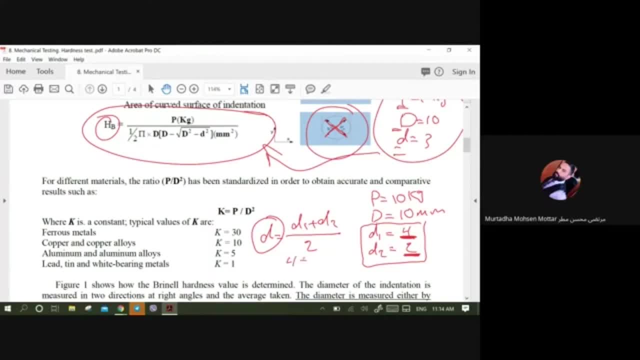 Like this. Now, like this: 4 plus 2.. You say 4 plus 2 divided by 2.. 4 plus 2 will give you 6 divided by 2, which is 3.. This is D small. 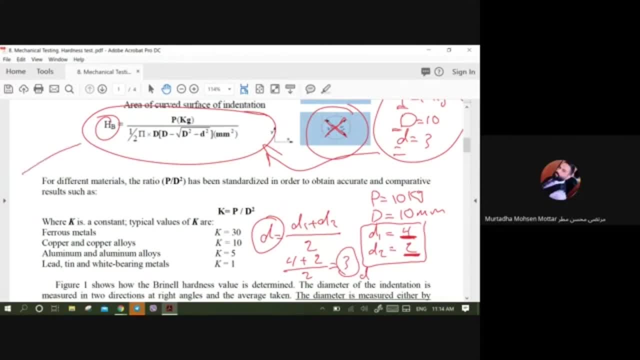 This is what you use in this law. This is what you use in this law. So if you subtract D1 and D2, you have to put them together and divide them by 2.. Now, of course, this is a step. 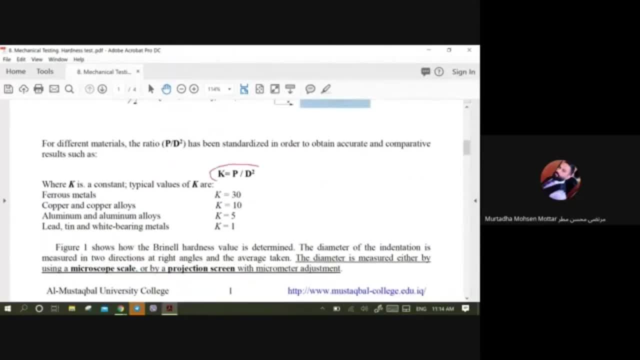 What is K? Now someone will ask: what is K? K is a constant. See: K equals P divided by D squared. Sometimes it doesn't give you the power. I mean it doesn't give you the power, It only gives you D, small. for example, 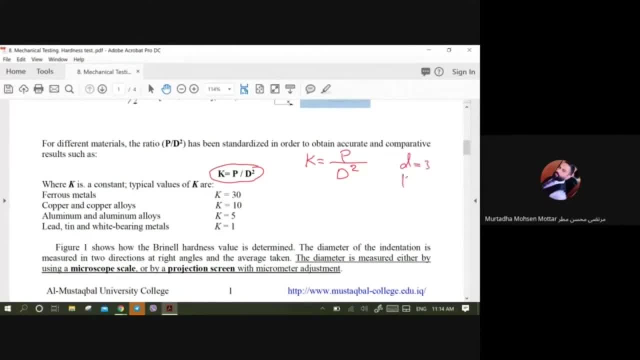 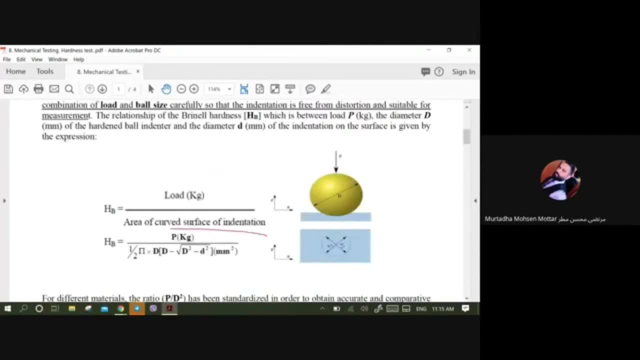 It gives you 3.. And K tells you, for example, K is 30. So you know that this is your law. This is your law. You must have a law, You must have a power And you must have D capital. 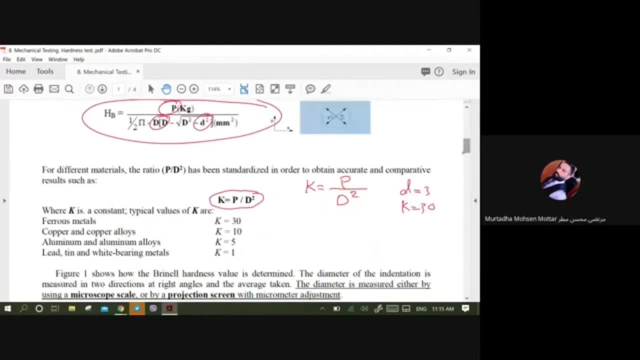 And you must have D small So that you can subtract them Here. it only gives me D small. So what do you do? You have this law: K, P divided by D squared. You know that if you don't get the D capital, if you don't get it by question, 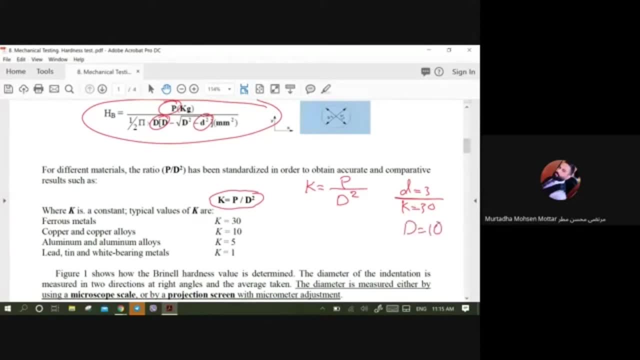 you should give it 10. Because I told you that it usually doesn't get 10.. And if you get its value, then you use it. Usually the D capital doesn't get 10. Because K- look K- is constant. 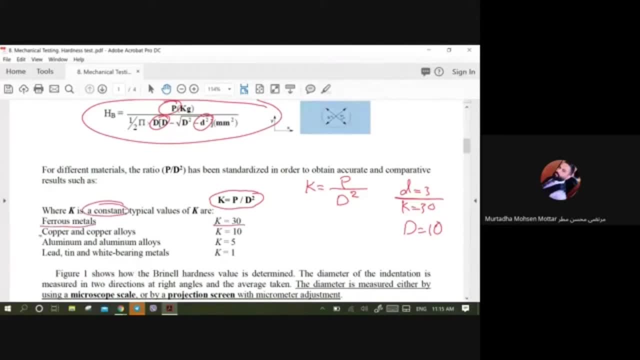 K is constant. For iron materials, its value is 30.. For copper and steel its value is 10.. And if you get the question, I'll give it to you. For aluminum and steel, its value is 5.. For bullets and bullets, its value is 1.. 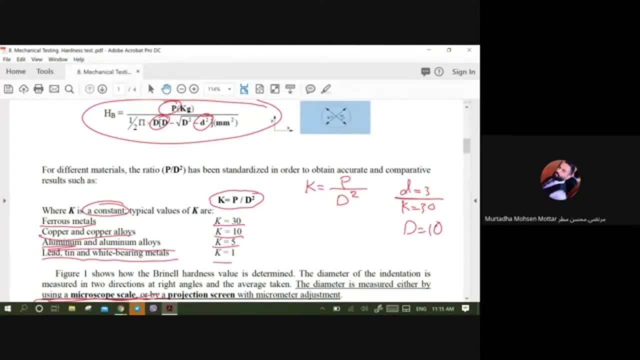 So now, what do I do? I'll give you, for example: its value is 30. So it means for iron and steel its value is 30. So you say 30, what do we do? P divided by D squared. 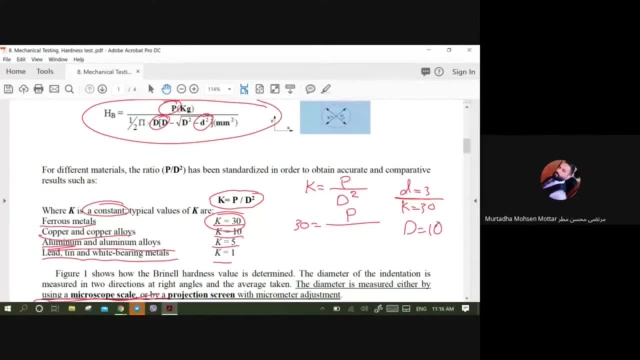 What is the value of D 100.. 100, exactly 10 squared 100.. So now, if you multiply the two sides, you'll get L. P will be 3000.. This is the value of P. 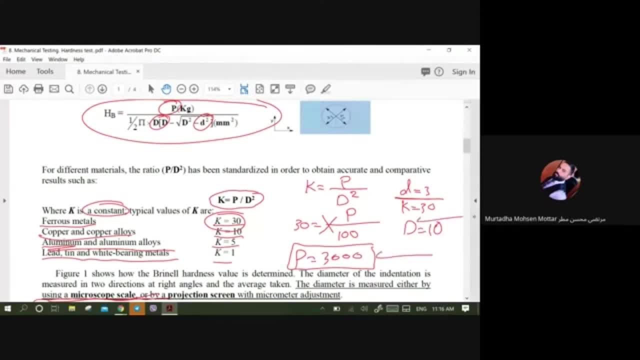 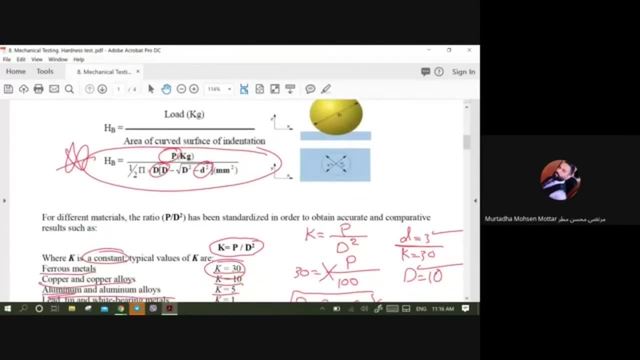 Now you have the value of P as information And D as information- the capital- And D small as information. Therefore, you'll be able to deduce the value of H brinole. I think it's possible that Sean will complicate the question. 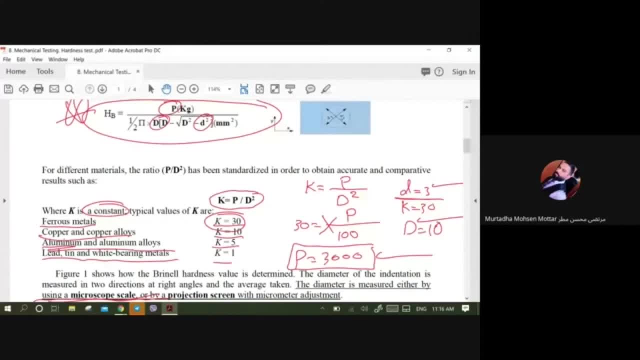 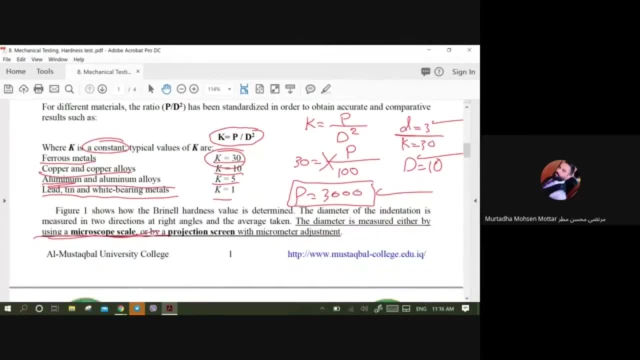 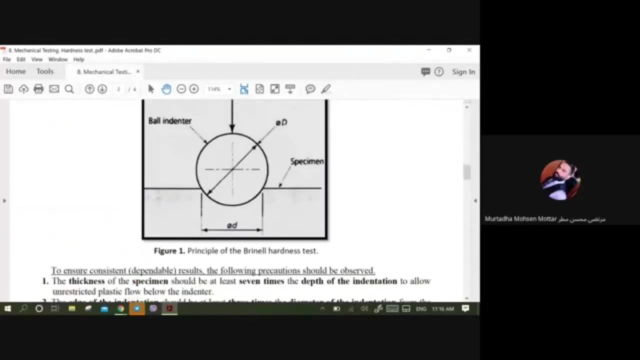 So he gives you the K and tells you to deduce the value of hardness. Now, is there a question here or not? Is it clear? It's clear, sir, it's clear. I see, Look, this drawing represents what. 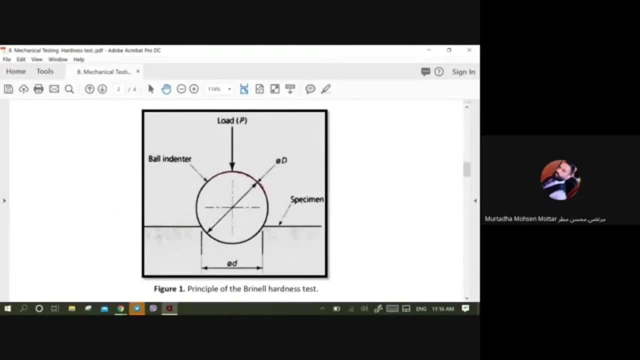 You have this body, this ball that is used. This drawing is required, students. This is the ball And this is the body that I'm going to draw like this. This is my sample, As you can see, I count the ball. 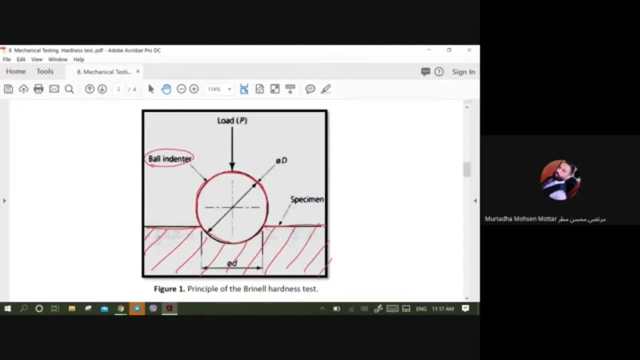 I call it the identar. Remember, I told you the identar a little while ago And this is the specimen. This is the tool, identar, And the specimen is the sample. The sample, This phi, is the diameter of the ball. 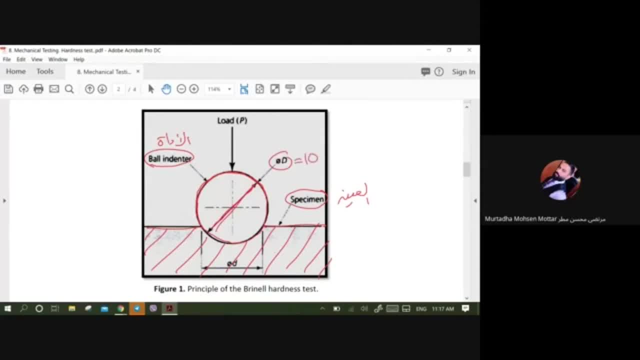 Which we usually said wouldn't be 10.. And here is the load. This load is different. This is the load, The load Or the weight, Or the force Which is the origin of the surface, And you count the radius of the effect. 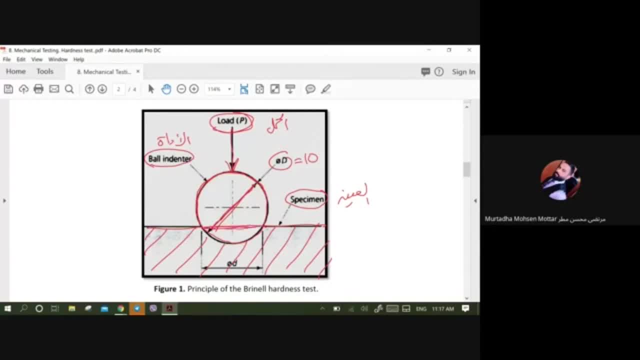 Where is this effect? How much does the ball roll? This is here. So this is the effect. If I want to know from above, I see it in a circle. Of course It has a certain radius, Which we said is d small. 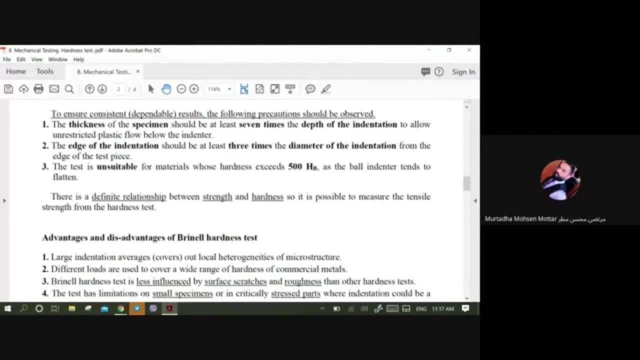 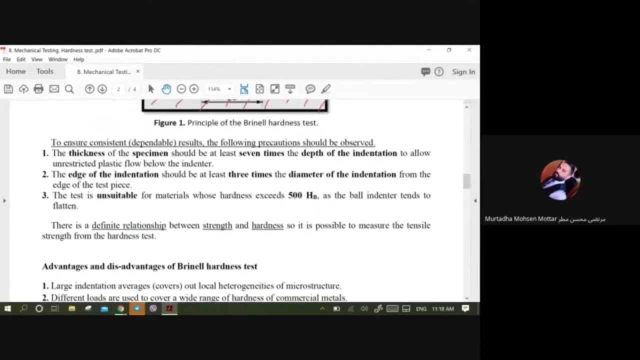 This drawing is required. Now we have this method. It has what Prequations? And it has advantages and disadvantages. What? First of all, it has equities And it has benefits for this method. Of course, Each method has benefits and equities. 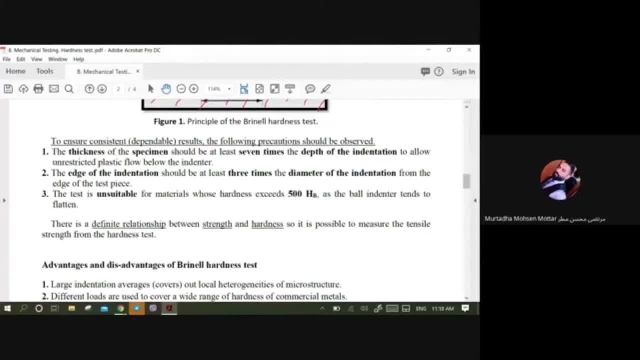 Look, In this you have three very important points. These points It can tell you to count, It can tell you if it's right or wrong, It can tell you these gaps. So you have- Look, I say- prequations. 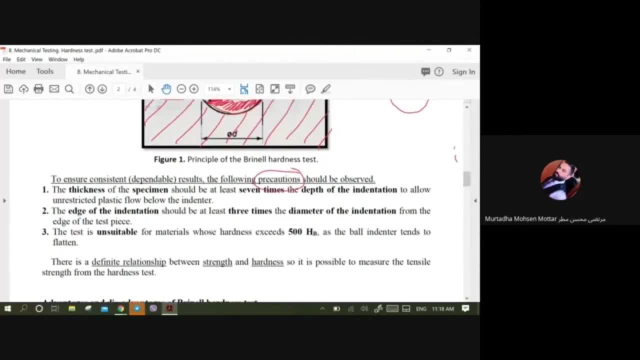 What does prequations mean? Prequations Now, what are prequations? Or the things that are taken into consideration in this test? To know what the results are dependent on. I mean, when I depend on the results, the results are not dependent. 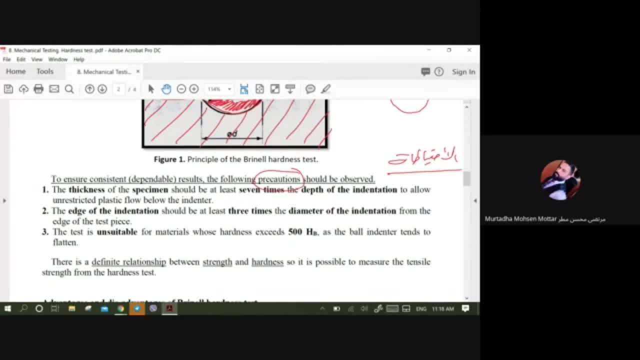 There must be things that I take into consideration. What are these things? If you focus with me These points, It is preferable to write them in Arabic next to you. It is preferable. It is preferable to write them in Arabic next to you. 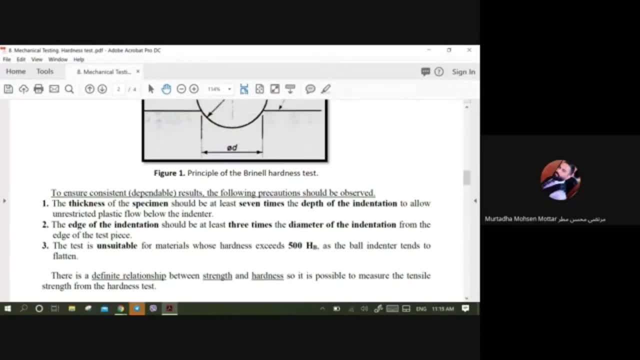 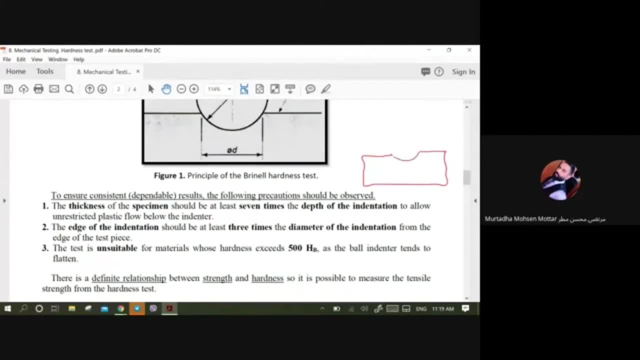 And you draw the drawing too. So, for example, this drawing itself, you draw it Here, for example- This is a sample, for example, And a ball fell on it. It left this effect, This effect, So this sample has an effect on it. 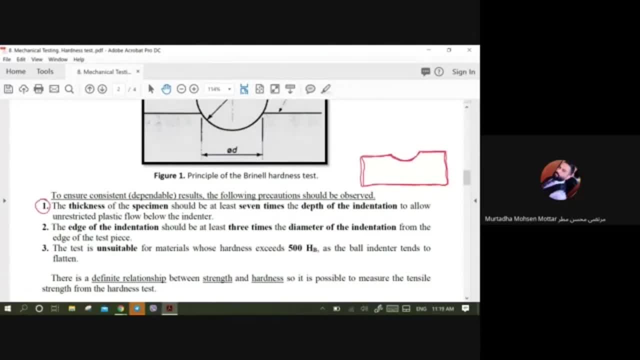 So now I come to the first point. The first point, What do you say? The thickness of the specimen should be at least seven times the depth of indentation. I mean, at this first point, The thickness of the specimen should exceed seven times the depth of indentation. 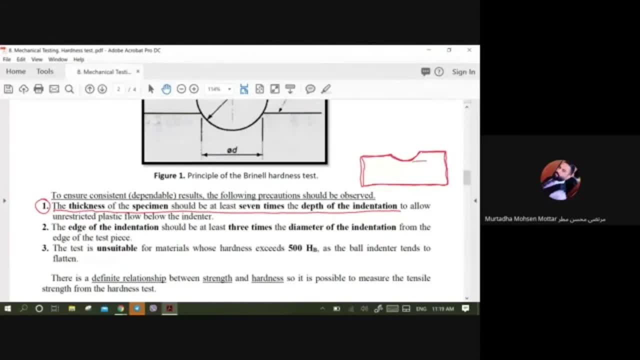 Where is the depth of indentation? Depth of indentation: Look, this is the depth of indentation. This distance is the depth of indentation. So, the thickness of the specimen, This is the thickness of the specimen. This is the thickness of the specimen. 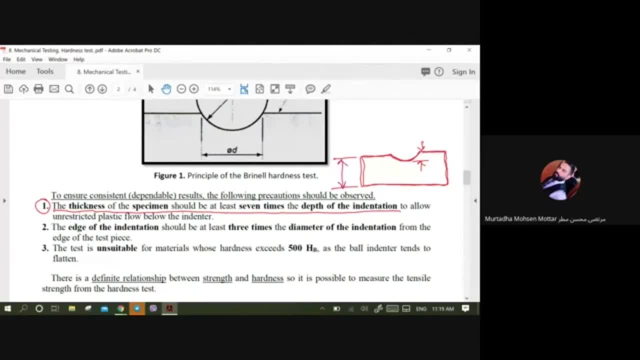 I said the thickness of the specimen should exceed seven times the depth of indentation. Let's assume that the depth of indentation is one millimeter, So how much is the thickness of the specimen? What is that? What is the depth of indentation? 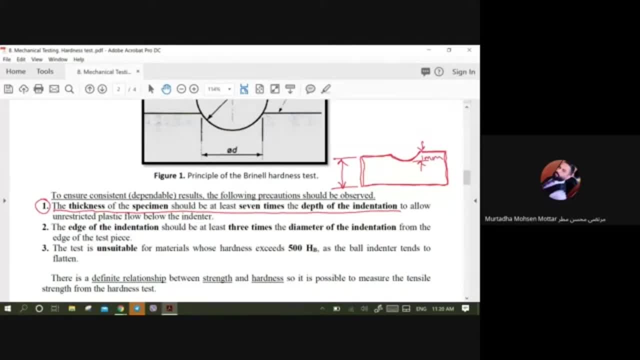 This is the depth of indentation. So how much is the depth of indentation? Depth of indentation I mean Depth of indentation, Depth of�school nitrogen. I mean it is less inンドation, the thickness of neutrinos which is less than the thickness 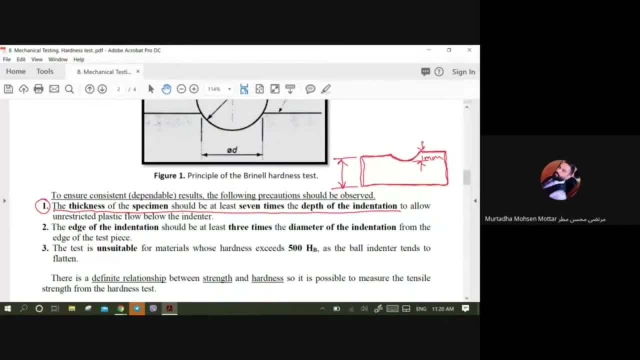 of thin MOC. So how much is the thickness of the specimen? What does that feel of this contaminant? 7 examples of depth of the effect. The thickness of the sample must exceed 7 examples of depth of the effect. This is the thickness of the sample. 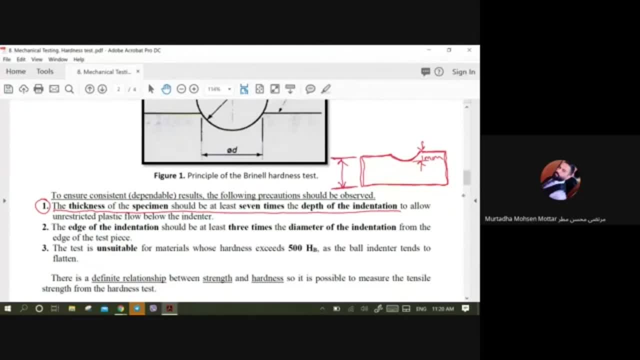 And this is the depth of the effect that the ball leaves. So let's assume that the depth of the effect is 1 mm. How much is the thickness of the sample? 7, 7 and above, 7 and above, 7 and above, Not 8. 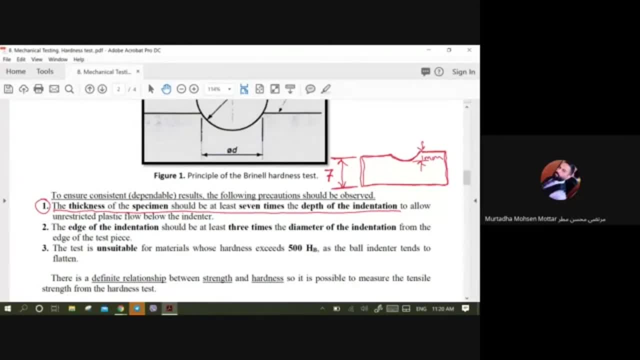 7 and above. I told you that the first point is that the thickness of the sample must exceed 7 examples of depth of the effect, So that there is no distortion of the sample. Why? Because let's assume that I have this base, This body, if I didn't leave it like this, in this shape. 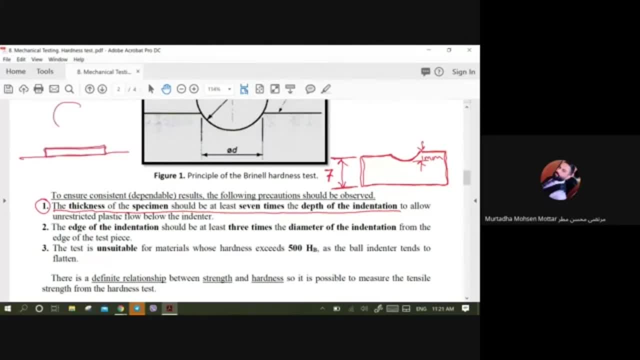 So this ball, when it falls, it can fall on it so that it reaches the end. here I mean, as if the material is distorted And therefore it will not measure its accuracy correctly. The thickness of the sample must exceed 7 examples of depth of the effect. 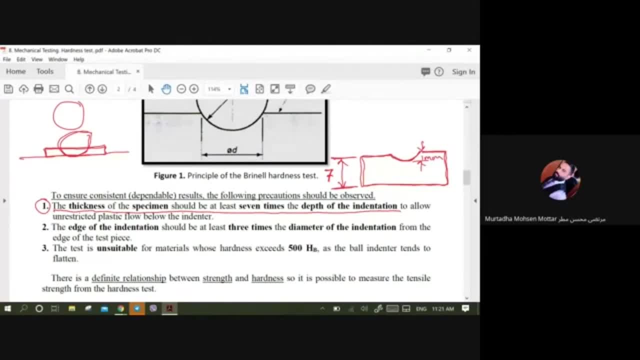 Did you write this point or not, students? Yes, sir, Write it. this is the first point. The second point: see what he says. The edge of the indentation. Edge means the end or half of the effect- Should be at least 3 times The diameter of the indentation. 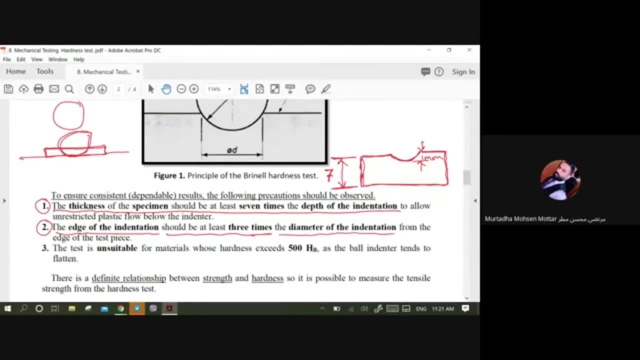 What does it mean? The edge of the indentation must be at least 3 times. Where is the edge of the indentation? See, if you want to focus on drawing, This is the edge of the indentation. Or this is the edge of the indentation. The indentation must be at least 2 times. 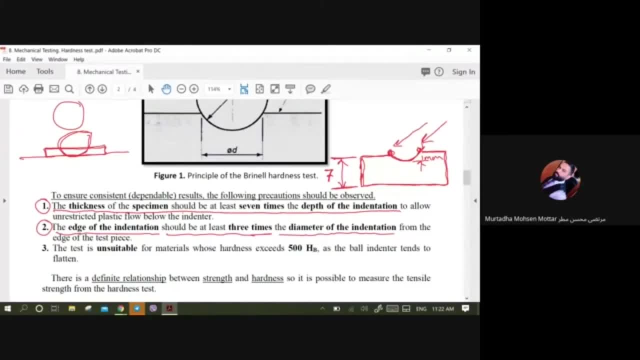 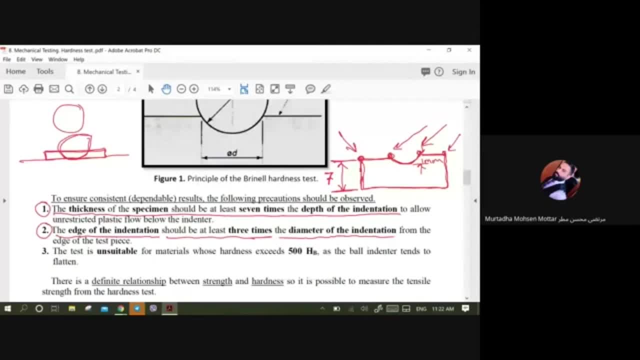 Or this is the second edge of the sample. So you have these distances. So it tells you that the edge of the sample must be away from the edge of the sample In order to increase 3 times the length of the indentation. See, this is the length of the indentation. 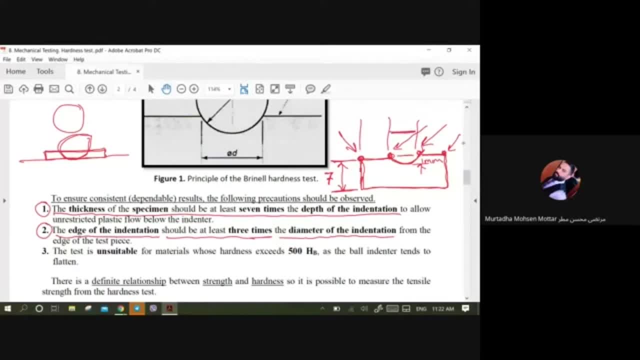 This is from here to here. This is the length of the indentation. So let's assume that the length of the indentation is 1 mm. So here, from this point to this point, How much does it happen? 3 times the length of the indentation. 3 times the length of the indentation. 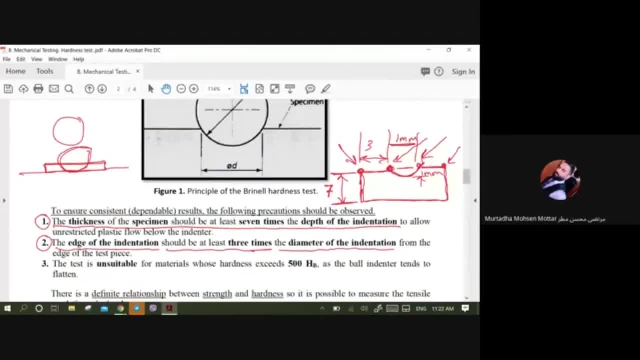 3 times the length of the indentation. So now you have the second point. To write it, You must keep the edge of the sample away from the edge of the sample. If you write it, You must keep the edge of the sample away from the edge of the sample. 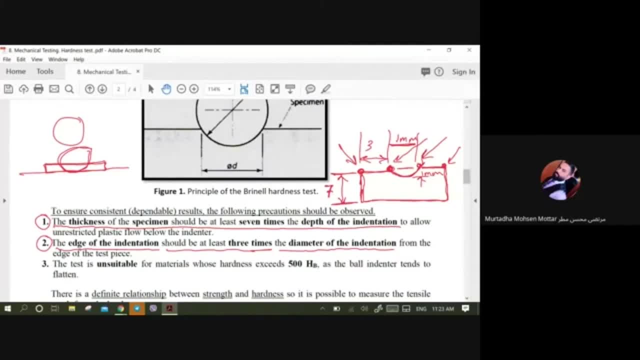 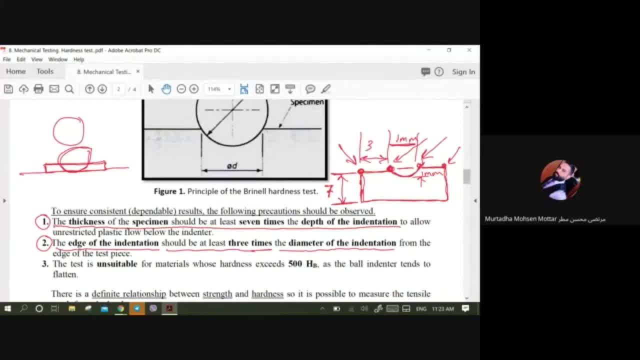 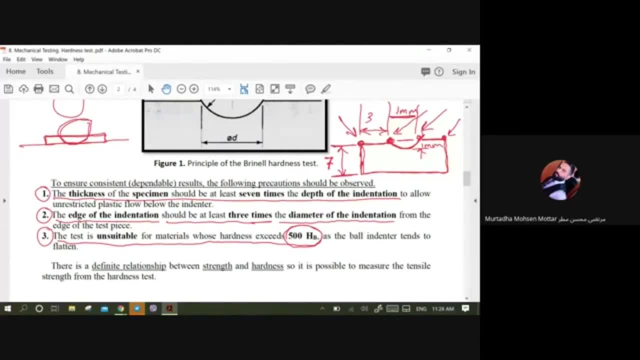 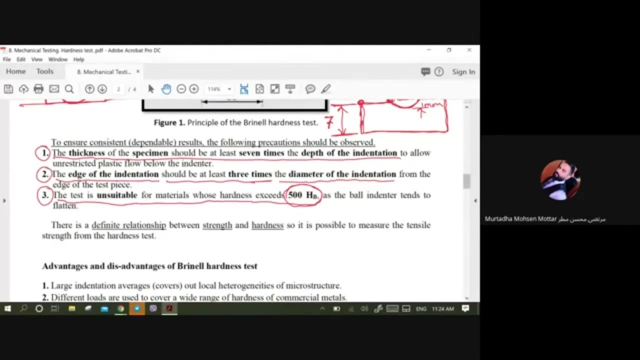 solidity 500 HB. I repeat: this test is not suitable for the material that its solidity is more than 500 HB. I repeat: this test is not suitable for the material that its solidity is more than 500 HB. Why? Because let's assume this material, this material. 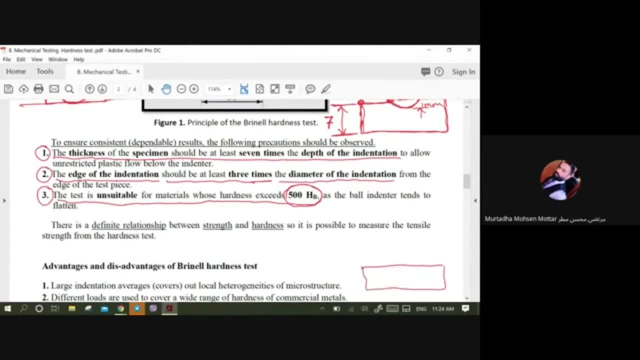 its solidity is more than 500 HB. orada الكرة هي أقوى. أعلى صلاة إلها كrants من كرة فبالتالي. لو كانت المادة أكثر صلاةب كرة فبالتالي. 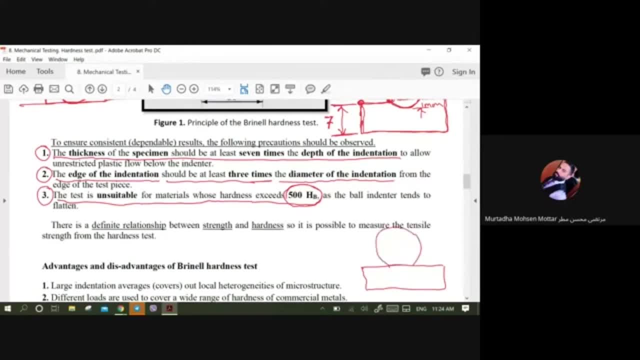 الكرة من lireح تسقط, كأن ما هي الكرة اللي تتأثر. تصبح سطح حفلات هالشكل كأنما تنبأش هي الكرة فبالتالي إنه هنا شوف يعني. 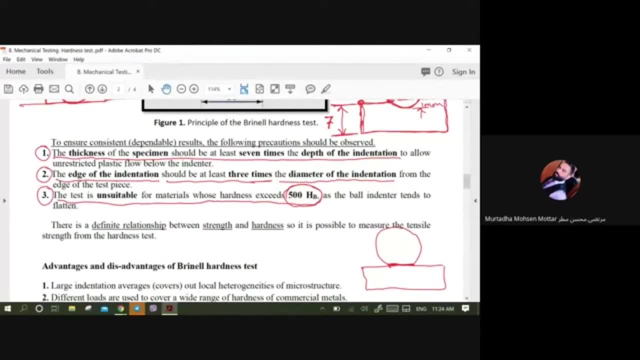 شعلسها. وهنا أنا لازم أستخدم طريقة ثانية. فهذا الاختبار غير مناسب that exceeds its solidity of 500, because if the material exceeds its solidity of 500,, 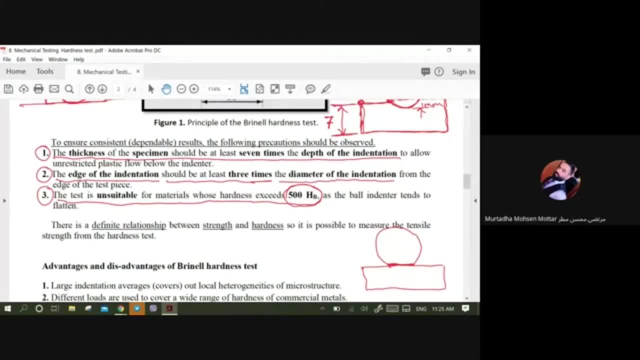 then the ball will not fall. not, the ball will stick to the metal. no, because the ball is what will be sold. there will be sales. so the third point: what do you say? this test is not suitable for the material that exceeds its solidity of 500H with hardness. 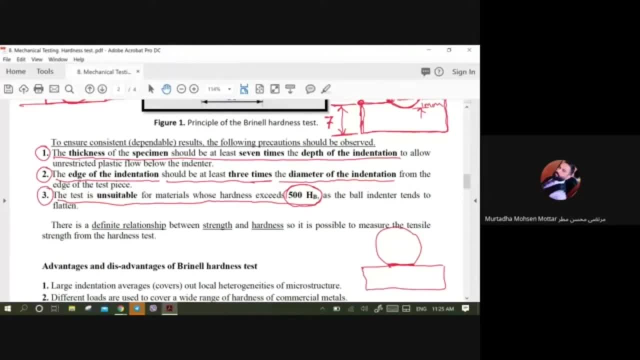 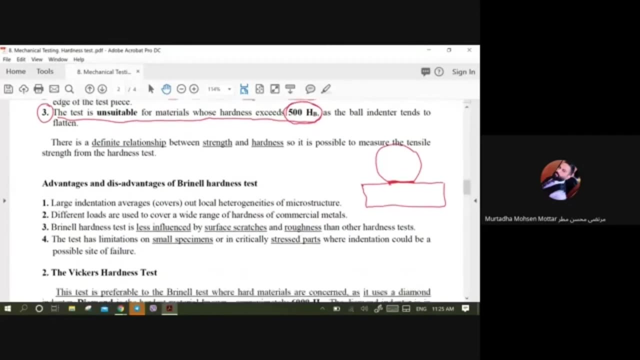 And now we have the three points. is there a question? Will I continue, my teachers? No, you continue your question. Now we have only the advantages and disadvantages and we will stop here. The second way: we will take it in the next lecture. 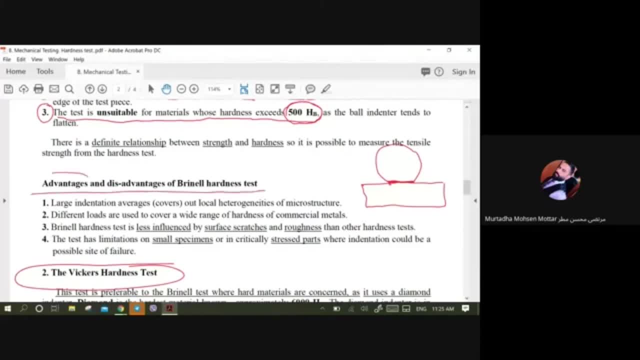 Here. you see, here the advantage means the benefits this way, and the disadvantage means the equal. here they are equal to the advantages and the disadvantages is equal to the disadvantages. here they are equal to the disadvantages and the disadvantages is equal to the advantages and the. 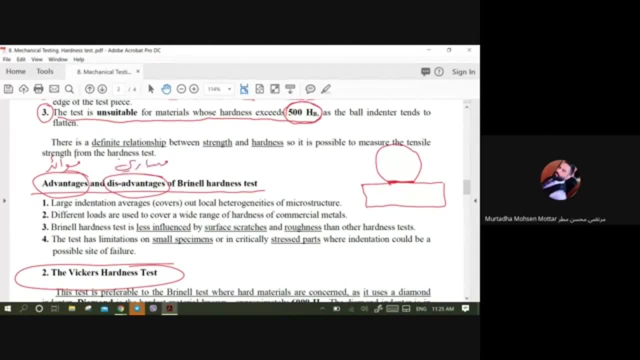 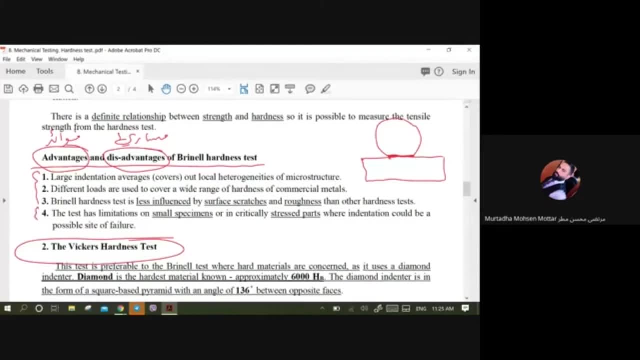 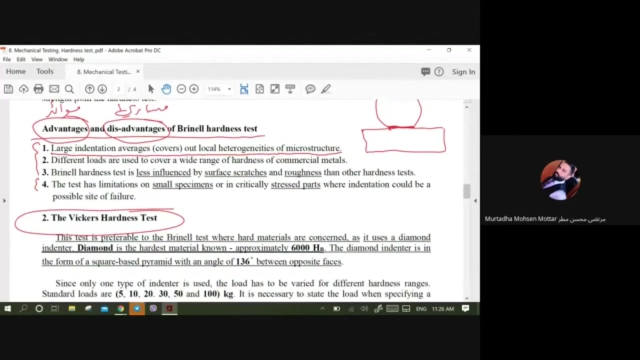 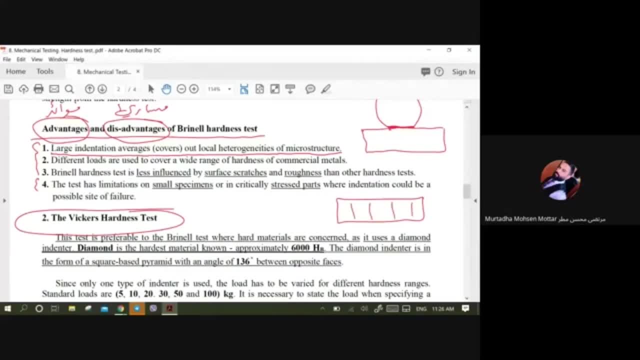 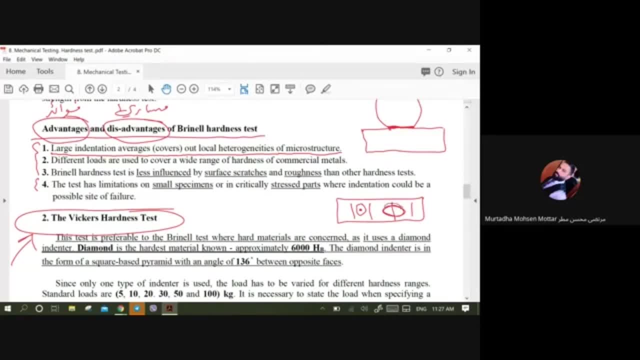 But this way the ball, because it is large, will cover a wide area of ​​matter. so it gives me an equation for what the matter contains, which means materials. This is the first point. so the first point says that the large effect covers a wide area of ​​matter. so this is what he means by it. 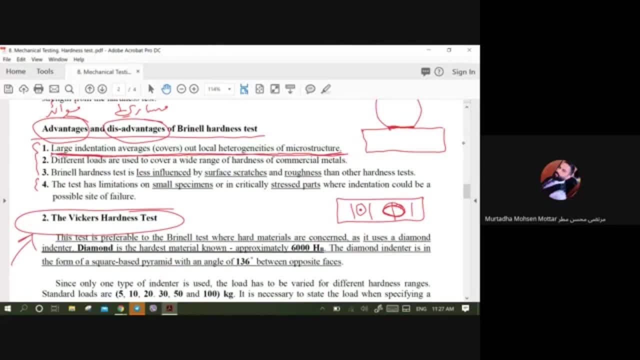 This is the first point. The second point says that different loads are used to cover a wide range of hardness of commercial materials. This means that different loads are used to measure a wide range of solidities of different materials. This is the second point. Different loads are used to measure a wide range of solidities of different materials. 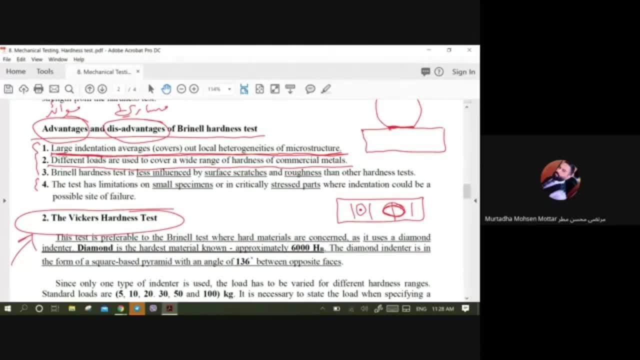 Different loads are used to measure a wide range of solidities of different materials, Because in this way the load is not constant. the load that I used, the power, the P, which we said a little while ago, is not constant, it is variable. 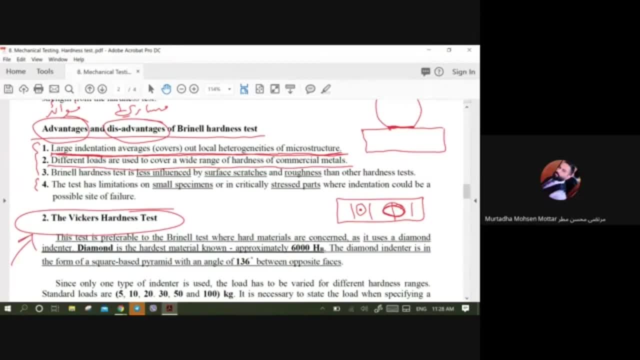 So I can change the load and use it with another material. This is what he means by it. Different loads are used to measure a wide range of solidities of different materials. This is the second point. There is a question about these two points. Do I continue with the third point? 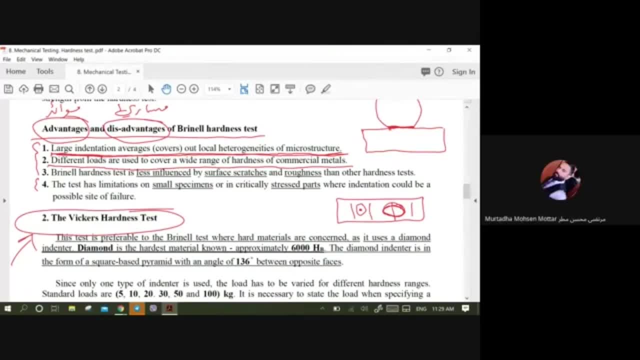 No, Saad, there is no need to continue. This is the third point. The third point is a brinal hardness test. It says that this method is less influenced by rough surface and softness. This is the third point. This method is less influenced by rough surface and softness. 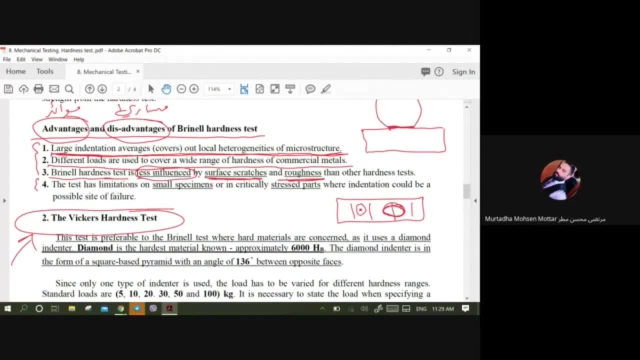 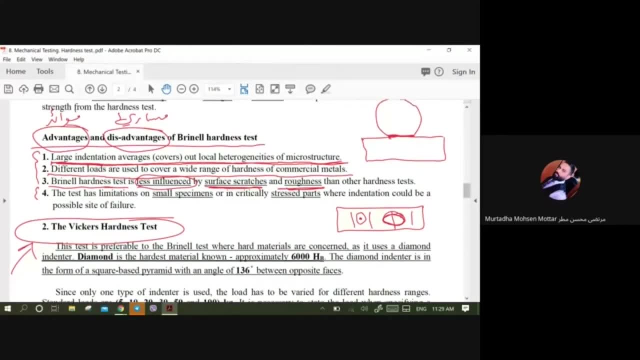 This method is less influenced by rough surface and softness. What does it mean by less influenced by rough surface and softness? I have other methods. There are some methods that I will discuss in the next lectures. What does it say? It says that if the material has softness or a surface that is not smooth, for example a mud, 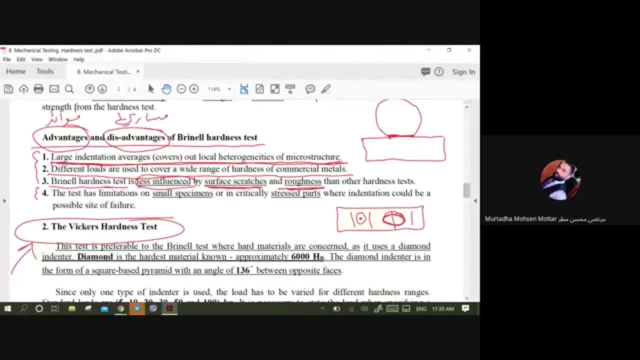 If the material has softness or a surface that is not smooth, it may fall on the mud. If the material has softness or a surface that is not smooth, it may fall on the mud. So I will not see the effect there. 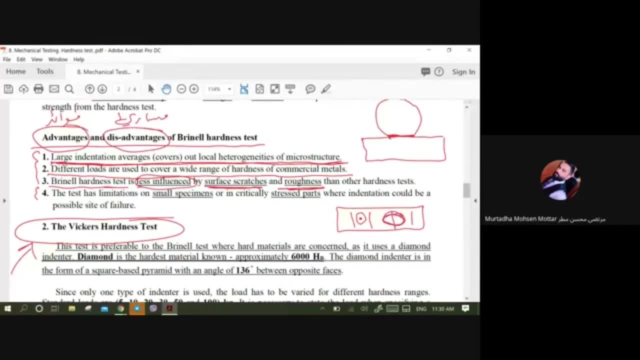 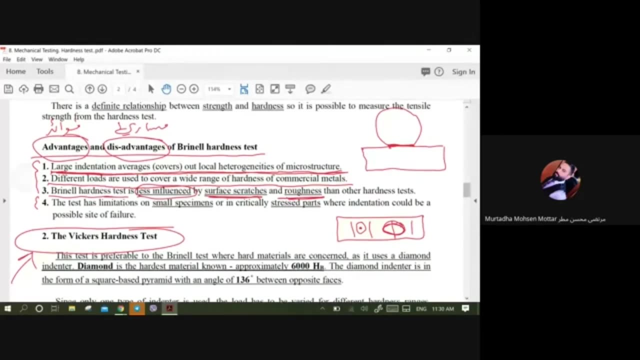 This method is a large ball, So wherever it falls, it will leave an effect, Even if it falls on the mud or on the mud, it will leave an effect. So this method is a large ball. This method is a large ball. 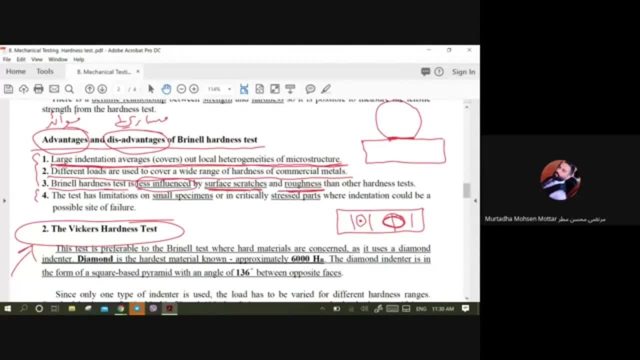 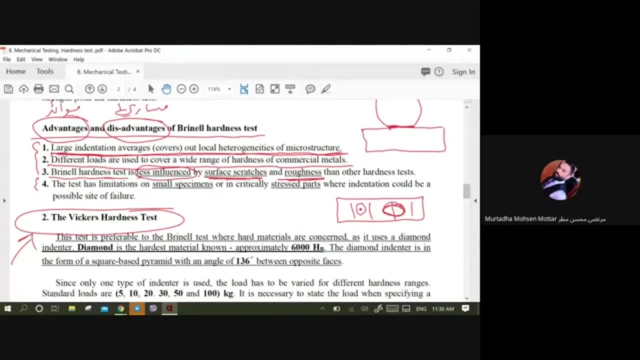 It is a 10mm ball, So this method is less influenced by rough surface and softness. There is another way I want to measure the surface, so I will do a grinding. I will do a grinding and then I will do a test. 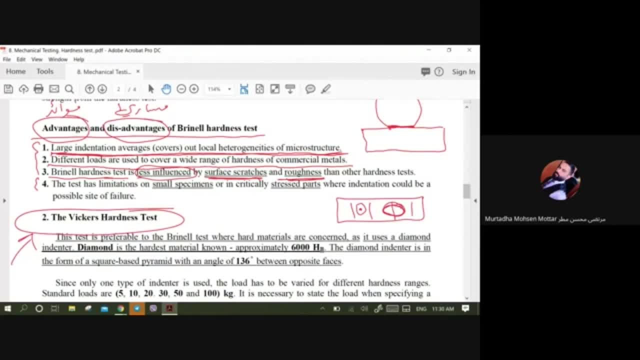 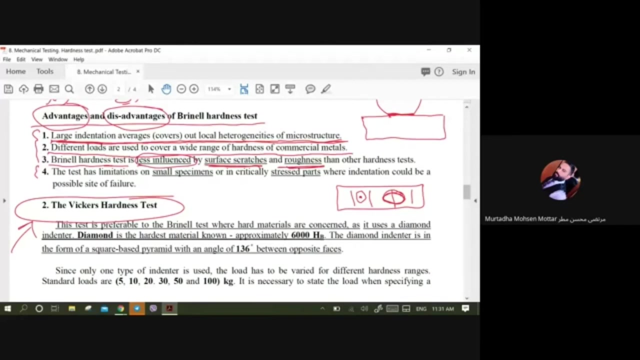 In the first test, Brno does not need to do a grinding and does not need to do polishing. This is the third point, which says that this test has less impact on the surface roughness and roughness. The fourth and last point is that it is a specific limitation or equal to this method. 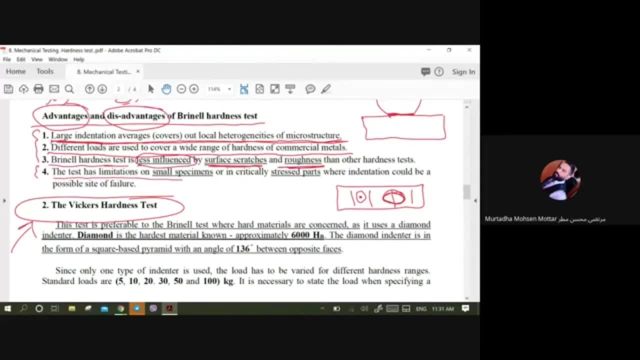 It says that the test has limitations on small specimen or stress bar. This test has limitations on small specimens and rough parts. The limitations of this method are the small specimen, the small specimens, the stress bar and the rough parts. You may ask: what are the small specimens and the rough parts? 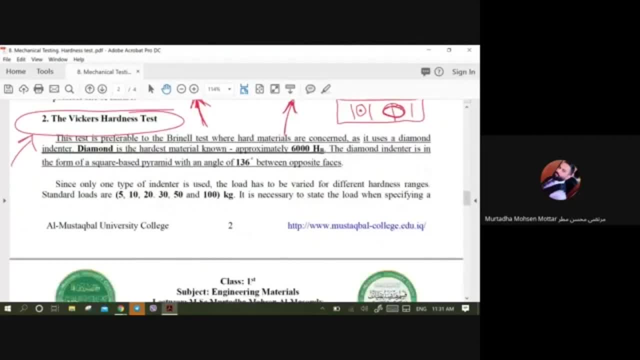 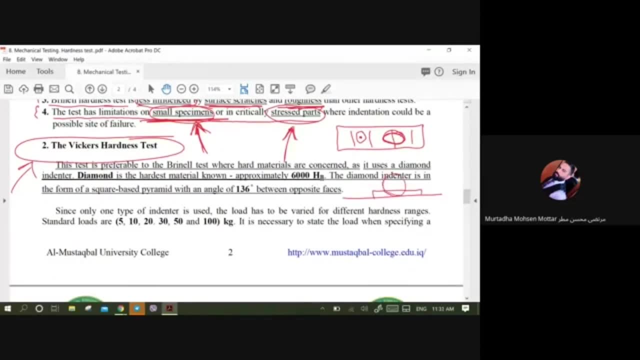 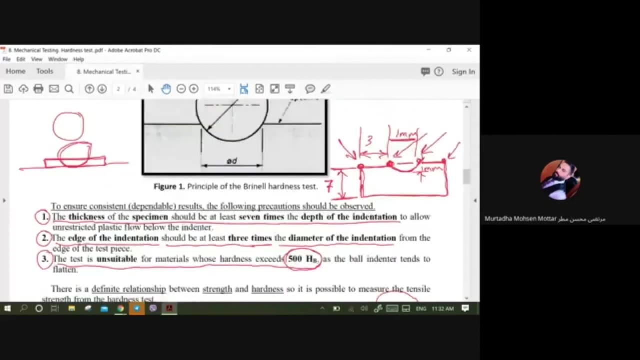 We explained the small specimens a little while ago. I told you that if you have a small specimen, the ball may pass through it and the material will fail and you will not be able to measure it correctly. Therefore, as I explained here, the thickness must be of a specific value. 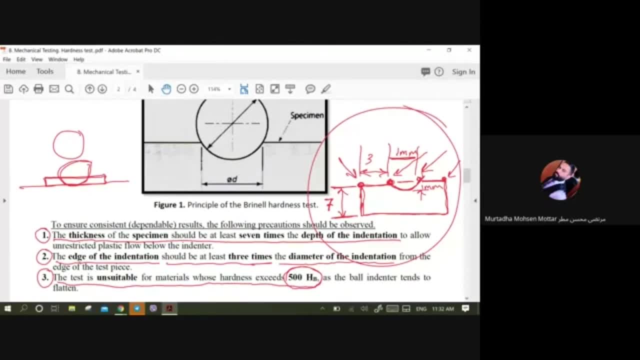 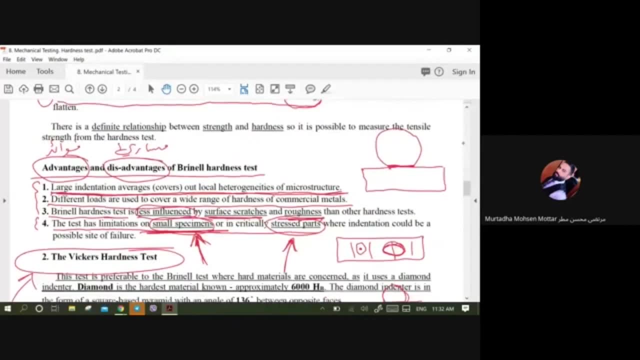 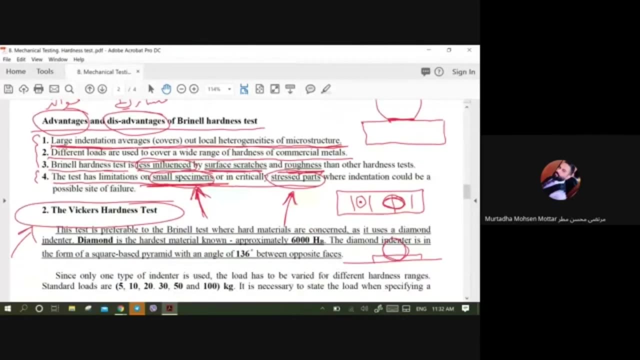 The thickness must be of a specific value, 7 or less, so that there is no distortion of the specimen. This is the third point. So this is about the small specimen. I told you that it has limitations for small samples. The stress bar, ie the rough parts, is what we mean by it. 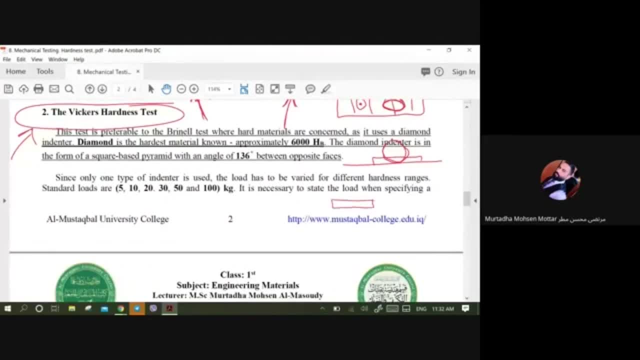 Suppose I have this kind of metal, This kind of metal. I made it stiff like this, I pulled it from this side and it will be more flexible. Of course it will be more flexible. So look at this kind of metal and this kind of metal. 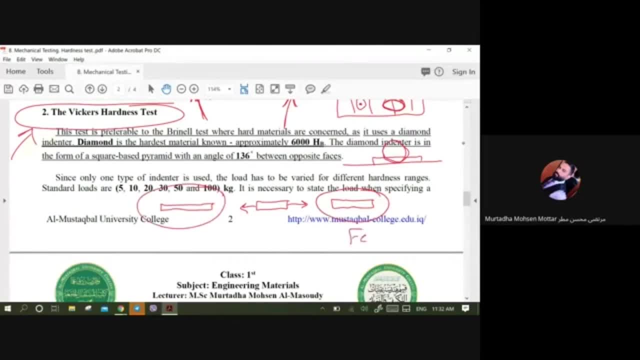 They are the same, They are two of the same. But to measure the strength of this part, the second part is hard. it is exposed to hard forces. so here the measurement of the strength is wrong. so to measure the correct strength, the body must be here without any external forces. 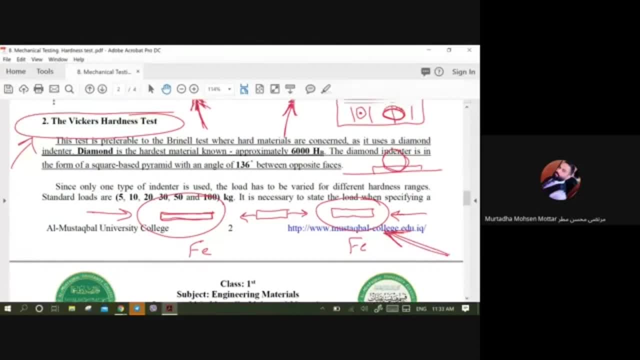 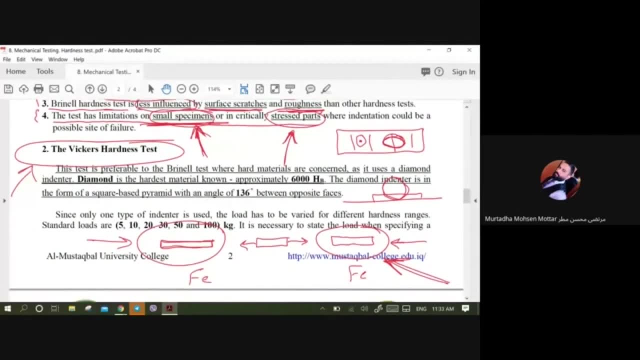 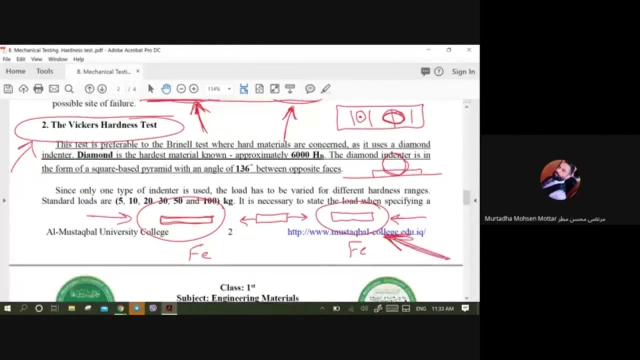 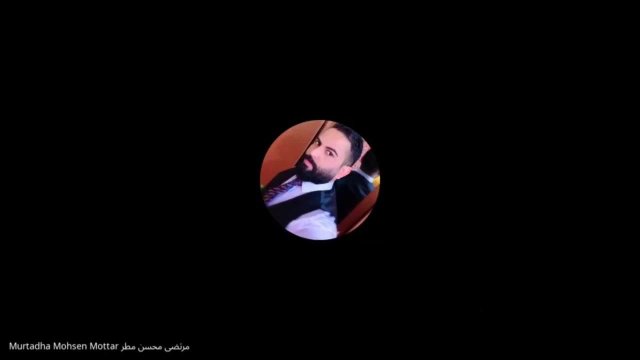 Or the material is not exposed to heat and other things. The material must be natural. This is the shape and the measurement of its strength. The specifications of this method are the small specimen and the hard parts, Because the ball may fall on a part exposed to heat. 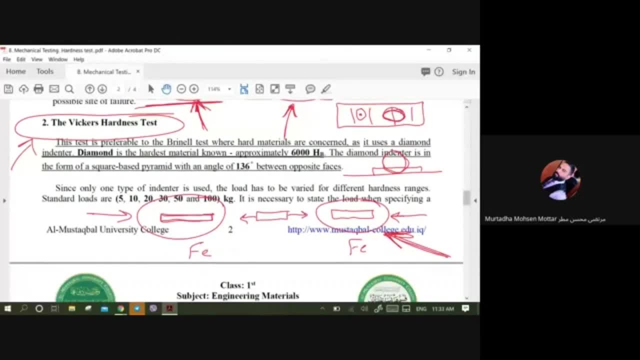 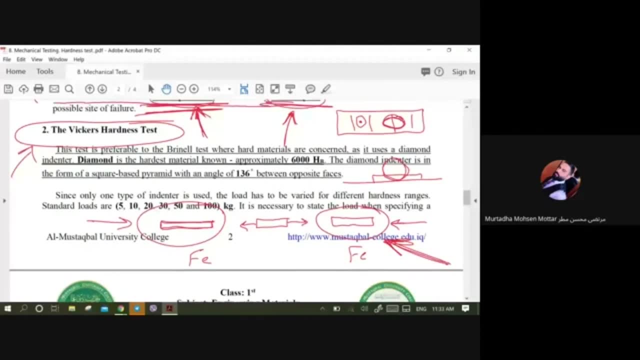 This is because it is exposed to hard forces or hard efforts. Therefore, it measures only the solidity of the area exposed to hard efforts. This is the result of a wrong operation. This is the fourth point, as I said, or the specifications of this method. 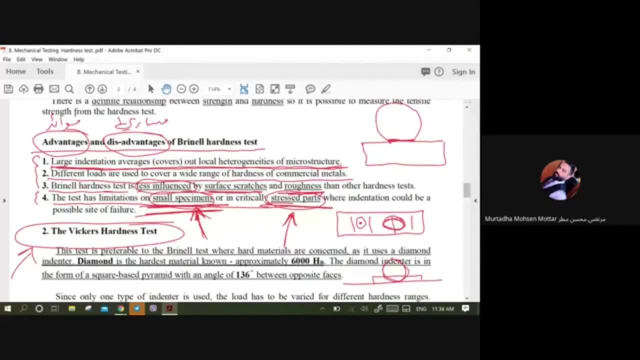 Of course, this is all for today's lecture. I will only talk about the first type of solidity tests. The rest will be continued in the next lectures. Any questions, Sir? just the fourth point, please. The fourth point. The fourth point is that this method has specifications. 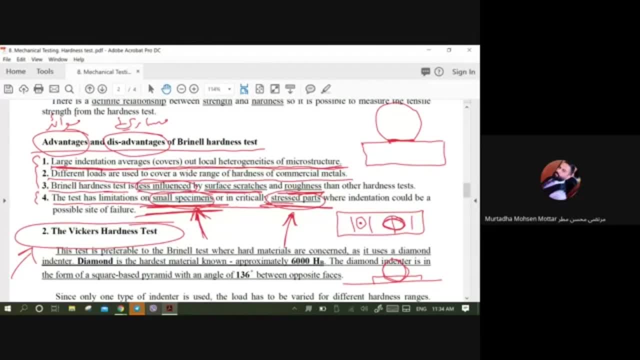 Which are the small specimens or the hard parts. This method has specifications: The small specimens and the hard parts. This is the fourth point. I told you that I will count them. You will count them. It may be that the material is correct or wrong. 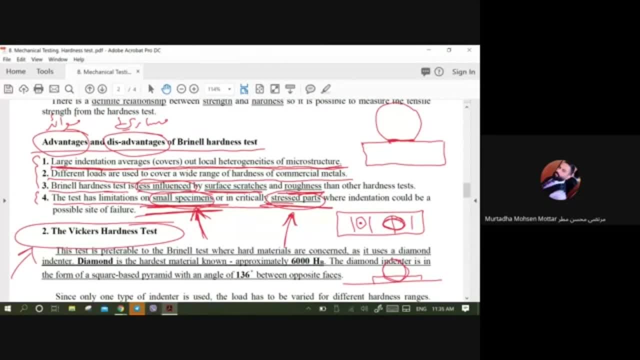 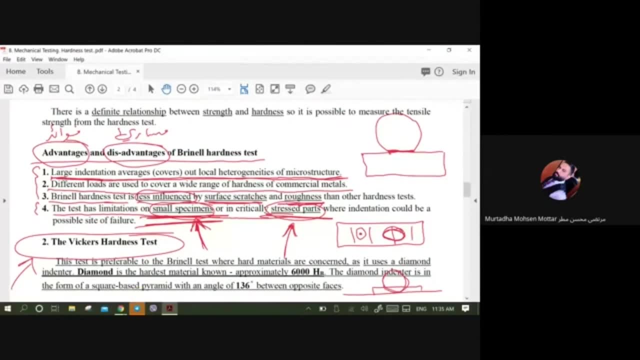 It may be true or false. These are two types of specifications: Specifications in the first type, I may tell you that this is the second type, Which is the Vickers. It is correct or wrong. You have to know. If it is correct or wrong, it is better sir. 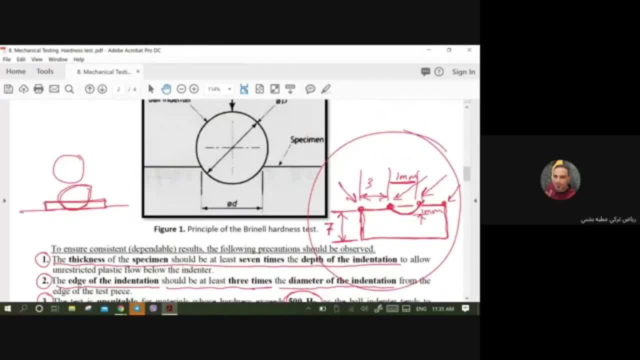 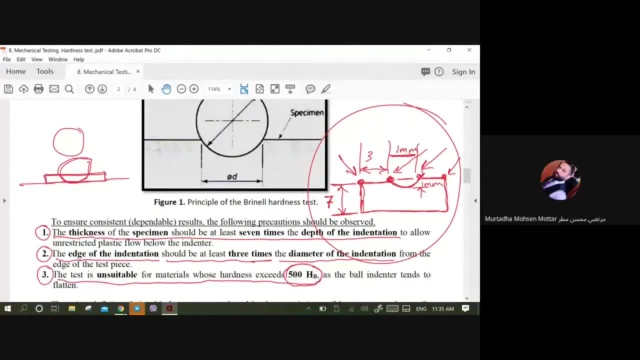 Because if it is correct or wrong, we have to memorize English And we are a little surprised that I did not learn English. Thank God for that. Correct or wrong is the same The sentence you find in front of you. If you see any change in it, it will be wrong. 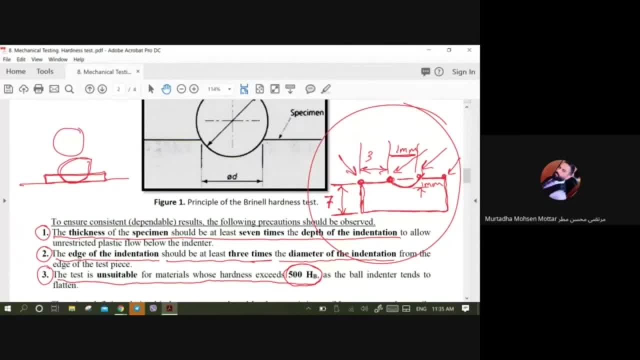 If it is correct or wrong, it will be correct. This is what I mean when I say true or false. The sentence is present, If I change it or leave it the same. If you see it, the same, of course it is true. 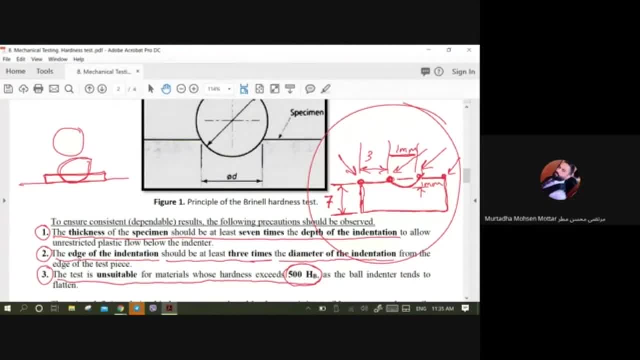 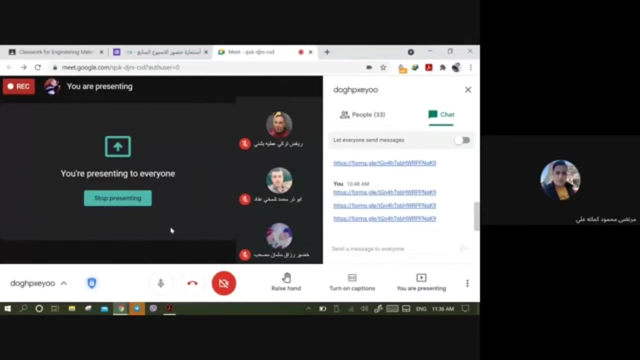 If it has a change, it will be false. Yes, There is a question about the lecture. Is this correct? There is a question about the lecture. We will record the lecture now. There is a question about the lecture. Stop recording. 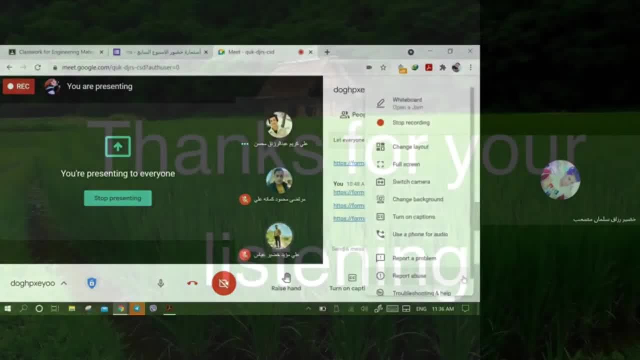 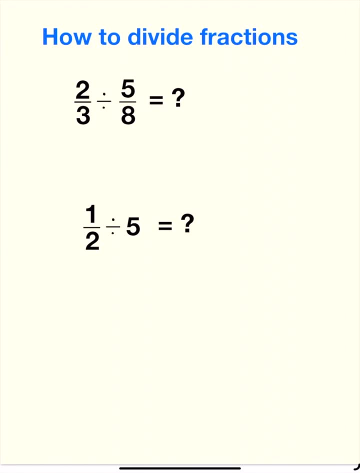 How to divide fractions. We have two problems here. Let's solve them. To divide by fractions, we need to multiply by the reciprocal, so the 5- 8 becomes 8 over 5.. This is equal to 2. 3rd,